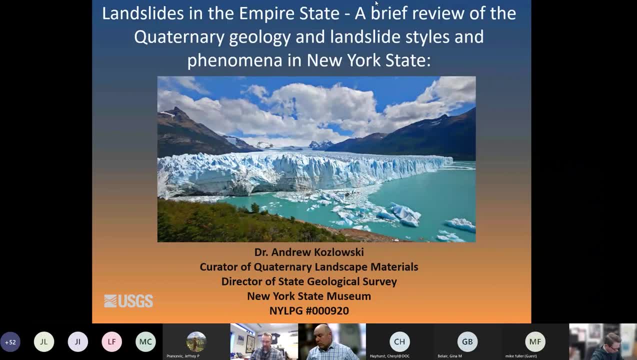 These talks will provide an overview of state landslide expertise, focus areas, product types and introduce some of the most pressing landslide-related problems that the state faces. If you'd like to have your state landslide work spotlighted as part of this mini-series, please shoot me or one of the co-organizers an email and we'd be happy to. 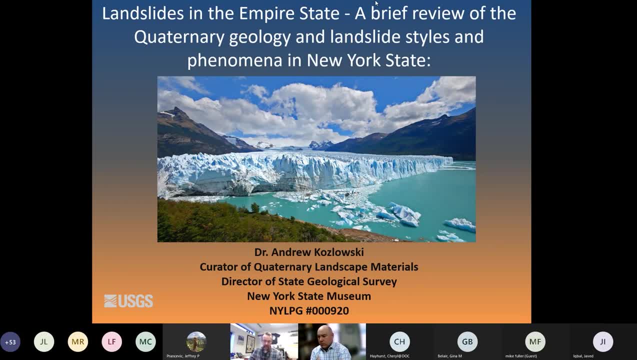 coordinate a date. Today we're joined by Dr Andrew Kozlowski. He's the director of the New York State Geological Survey and Geological Mapping Program, which is a bureau in the New York State Museum. He's a licensed professional geologist with an MS and PhD in hydrogeology. 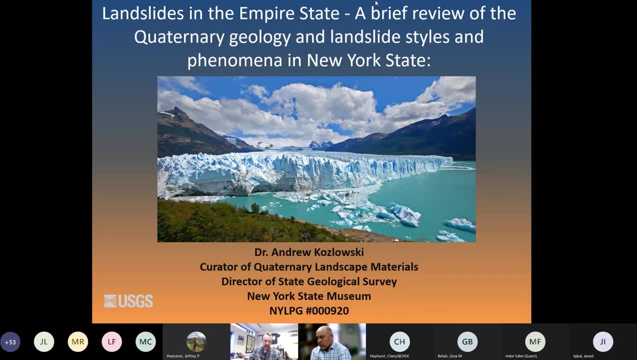 geomorphology and glacial geology from Western Michigan University. Andrew, thanks so much for joining us today. I'll go ahead and turn it over to you. Thank you very much, folks. It's a pleasure to be here and to present on some of the quaternary. 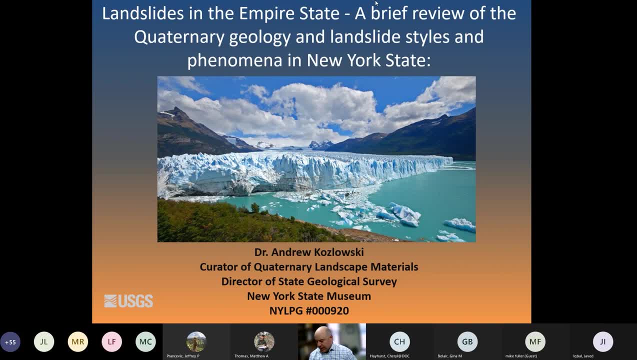 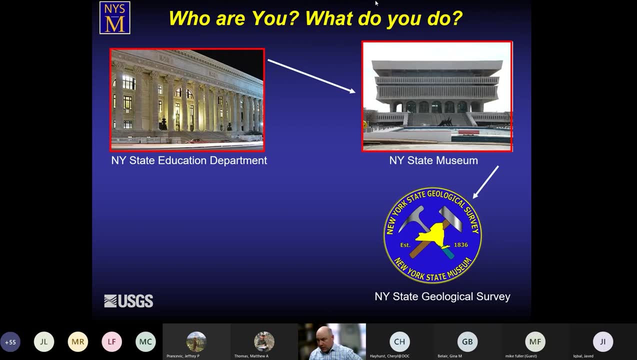 geology and landslide hazards we have here in New York State, Sort of just dive in. briefly, give an overview, because we are sort of an odd duck here in the sense of where our geological survey is housed. We are within the New York State government system. The geological survey is in the 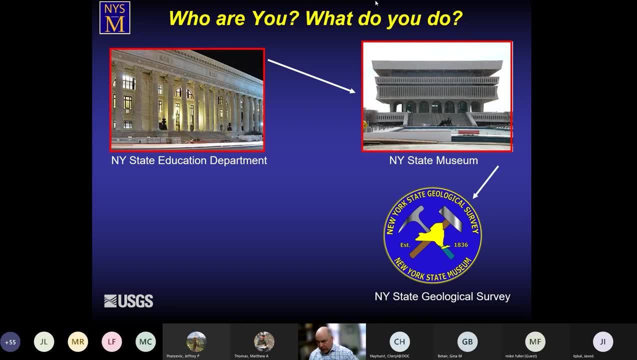 State Museum, which falls under the Department of Education, which, again, I think we're the only geological survey that's under Department of Education. I think Maine used to be, but they got smart and got out. So I'm a research scientist and I'm a director of the geologic survey and the 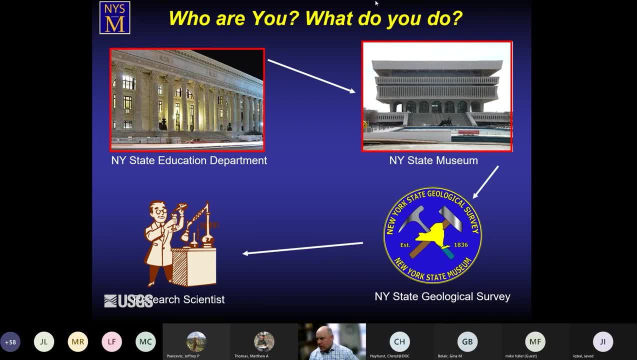 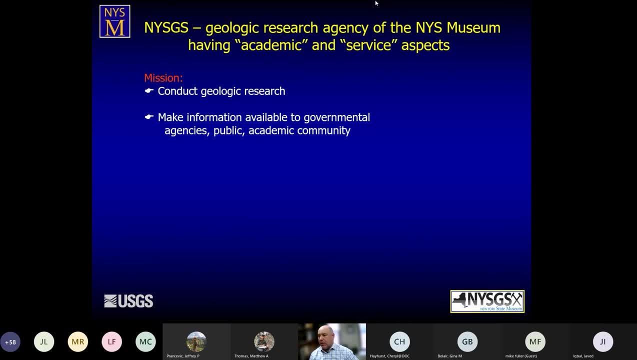 mapping program. So that's our organizational structure. We have academic and service aspects again towards the public: public information, education. that's kind of primary focus Again for again, health, safety, economic welfare, and we have a number of other things that we're. 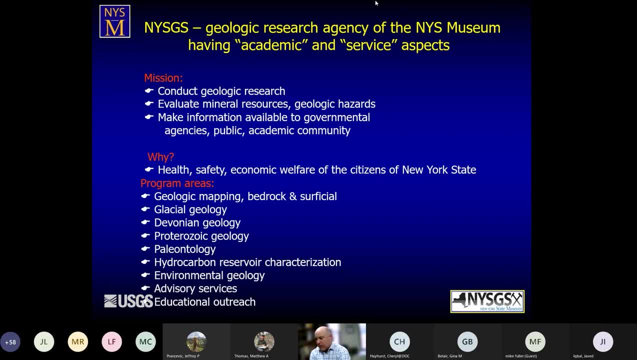 doing. We have a number of different programmatic areas which are in various levels of activity that we have going on. I'm primarily in my history with the museum as I've been here since 2006.. And again, I have a background in quaternary geology and geologic mapping. 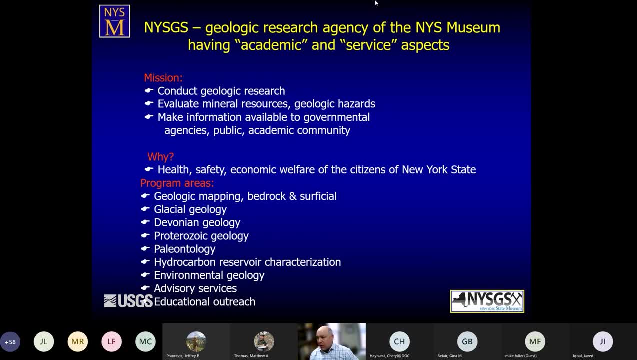 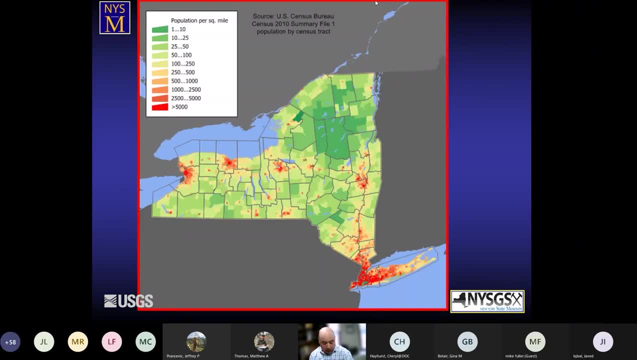 in this area. So that's sort of who is speaking and where we are. I just thought about this. when I was giving this talk When I was in graduate school in the Midwest, and I would tell people I was from New York, almost everybody would universally comment. 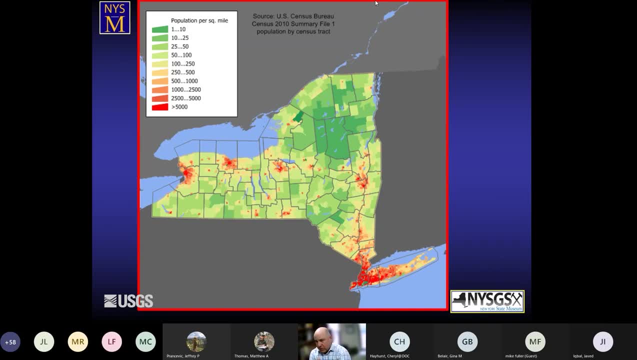 boy, I don't know how I could never live in a city that big. And I would say, well, no, I'm from New York State, And they go. yeah, it's got to be crazy with all those people, And so one of the things is just a population map. here The state show. 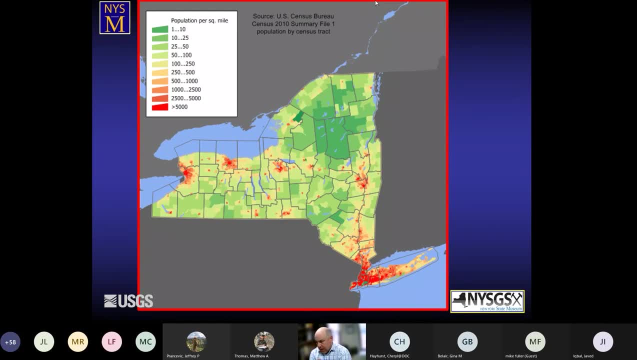 the populations for the state And the population is the highest down in the New York City area, down around Long Island of course, and high in the Hudson Valley over on the eastern part of New York State And then in a couple of the centers in upstate New York around Syracuse. 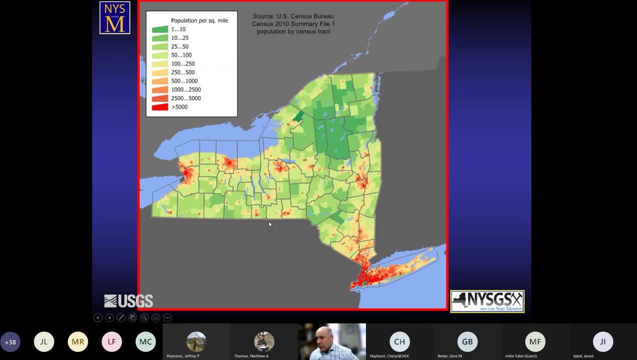 Rochester and Buffalo, But there are vast areas of New York State which are very desolate And very low population density, particularly in the northern part of the country here in New York State. So just an overview. It's a lot more rural than a lot of people think. So again an overview. 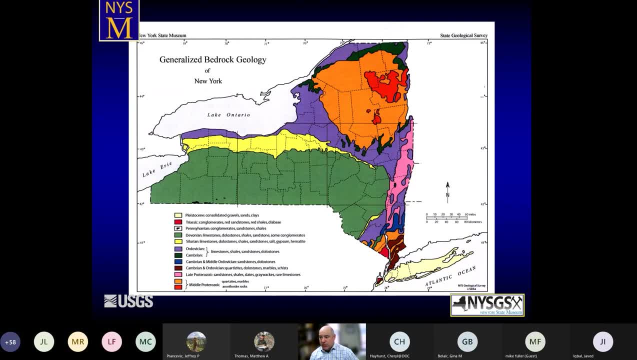 of our overall geology. This is very simplified. I'll just show another one of these later on. But again, most of the three quarters of the rocks in New York State are sedimentary Paleozoic, primarily Devonian and Ordovician in age, And then we have some very old igneous. 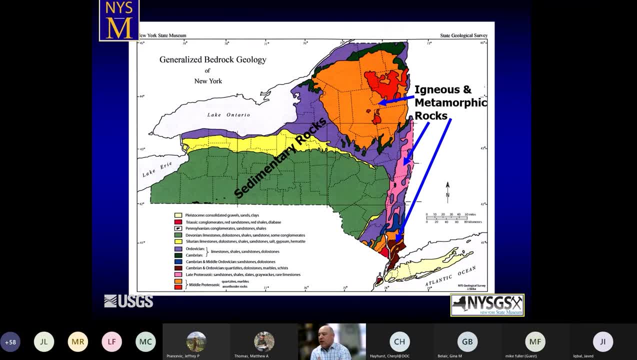 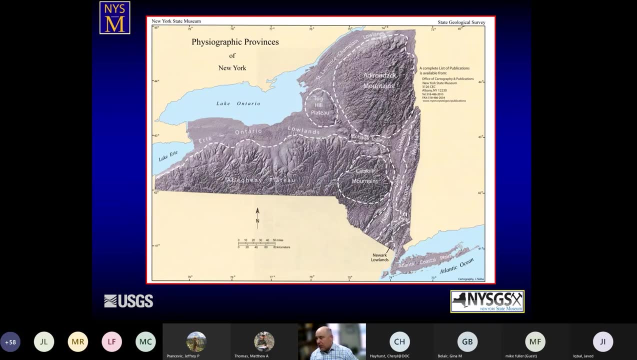 metamorphic rocks About 1.3 billion years old in the Adirondacks And some older crystalline metamorphic rocks down in the Hudson Highlands, down in the lower Hudson Valley. Physiographic areas in New York State Again: the Adirondack Mountains, the Catskill Mountains, Tug Hill Plateau, And then 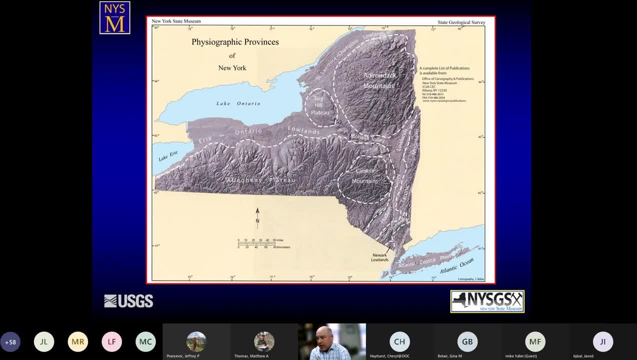 in a glaciated and fluvial dissected Allegheny Plateau And many lowlands such as the Hudson Lowlands and the Mohawk Lowlands and the Erie Ontario Lowlands, Sort of an overview of New York State, where we are And we call them. 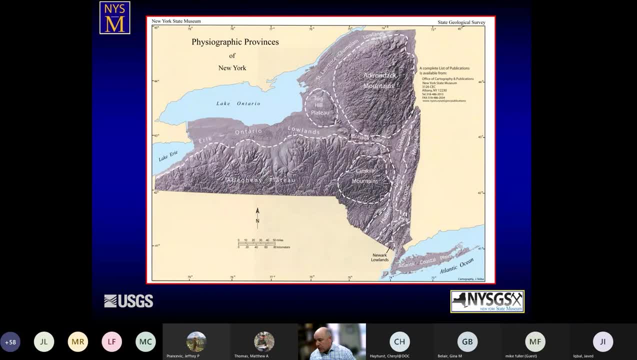 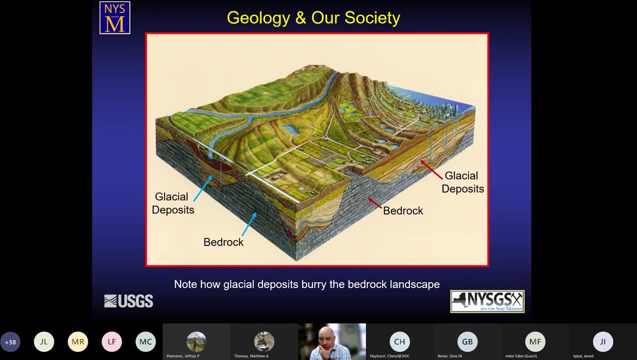 mountains out here, But for the folks out West it's just hills. So our program is based fundamentally on again sort of trying to address geology for society And again my emphasis is with the, the Quaternary or Pleistocene geology, And here, like many locations in the, in the 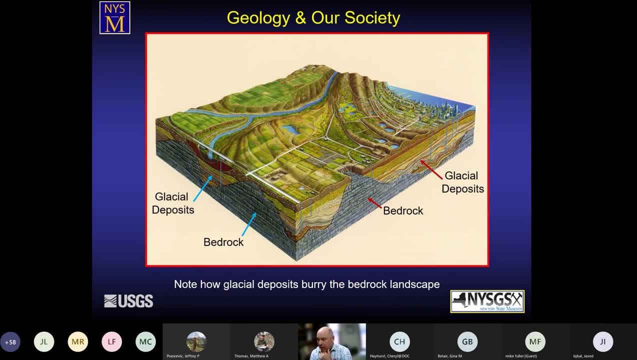 glaciated Great Lakes regions. a lot of our landscape is buried by glacial deposits. You know, we again we're, we're trying to figure out waste disposal, uh, how to protect water resources, how to protect ecosystems, uh, so on and so forth. so we've been taking and adopting a three-dimensional geologic 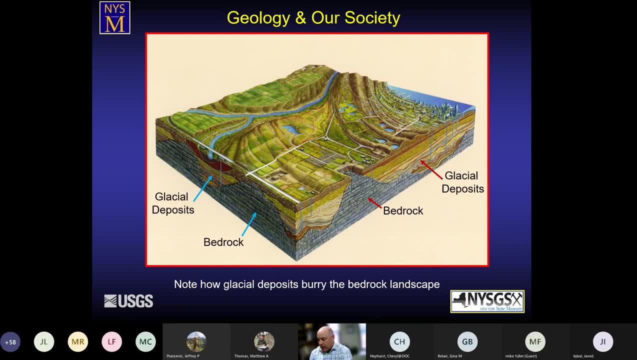 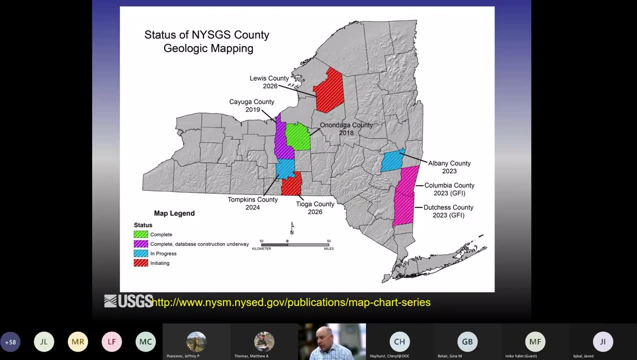 mapping uh sort of outlook on things in the last decade or so here at the museum. so a number of years ago, when landslides started to happen here and i was relatively new, i was talking with uh the time frame. we already had some mapping programs going on, but at that time i was talking 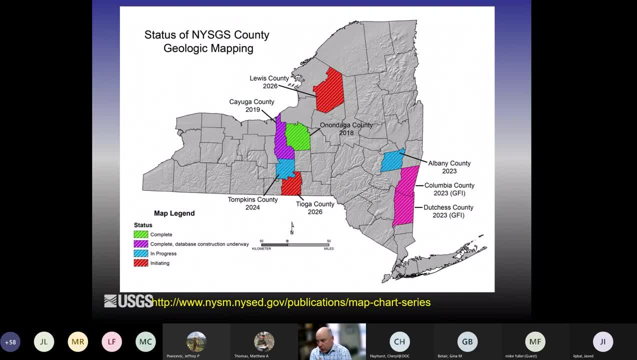 with francis ashland, with usgs, who was uh sort of working here in the northeast eastern first state, and i said: you know how do we go about tackling this landslide issue in trying to map them and figure out these elements? and he gave me some very frank advice and he said: don't even think about it. 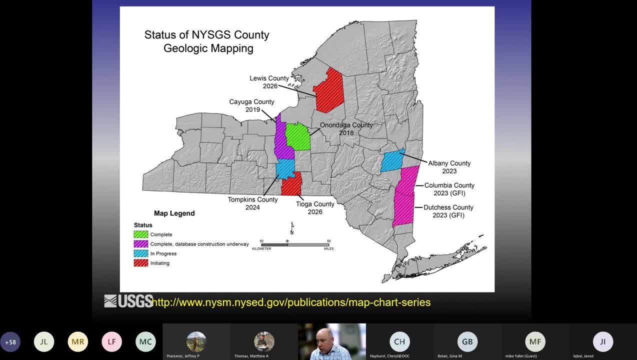 until you get your surficial mapping under control- and so that's where we've been for the last 10 years- is really diving in? uh, to do detailed surface geologic mapping. we map at a one to twenty four thousand scale on individual quadrangles and then we recompile them into 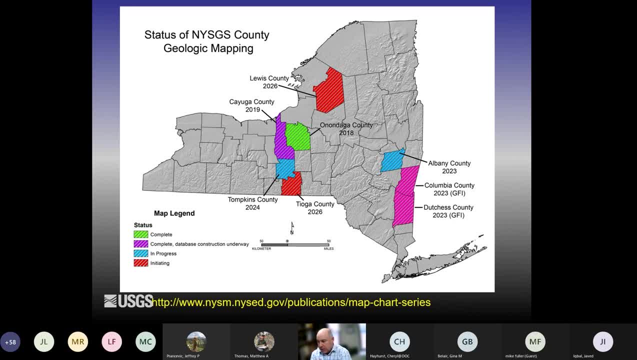 counties, uh, once they're done at better scales. so we have coverage for the entire state at scales of one to two hundred and fifty thousand, for both bedrock and surficial. but those scales are not really very helpful when you're talking about, like a county planning or a county engineer or health. 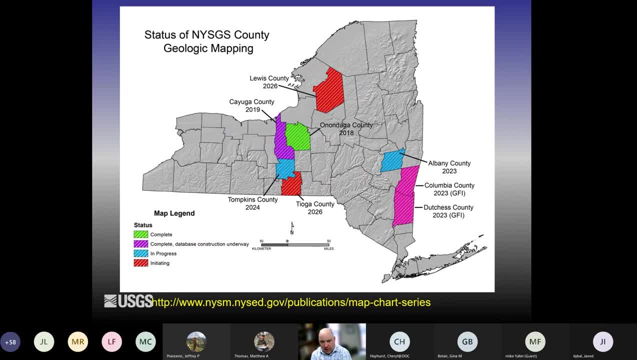 department that's trying to mitigate a landslide or better understand what the geology is. so we've been taking this approach and typically we're publishing these county-wide scales- maps at one to fifty thousand or one to one hundred thousand, which we think provides a scale for that still has some usability. but again we also have the individual detailed quadrangle. 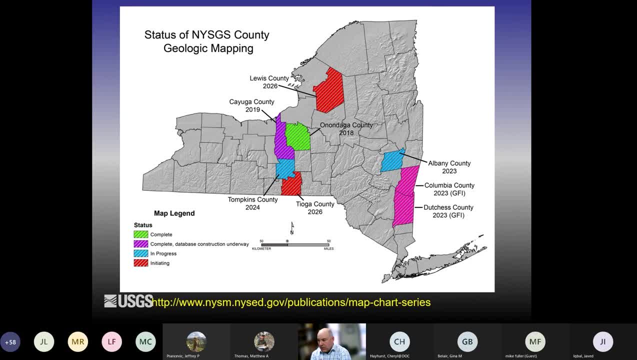 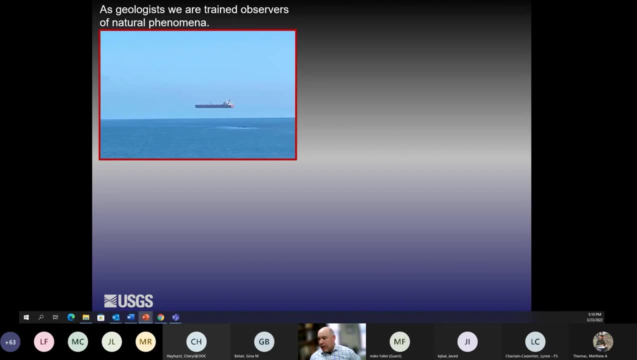 maps which are available, uh, before we compile the counties, when we're doing it- and this is just sort of an outlook overview of where the mapping we've been done and our maps are published for free, uh, via the all right. so again, it's one of the problems we face um as geologists across the board is that 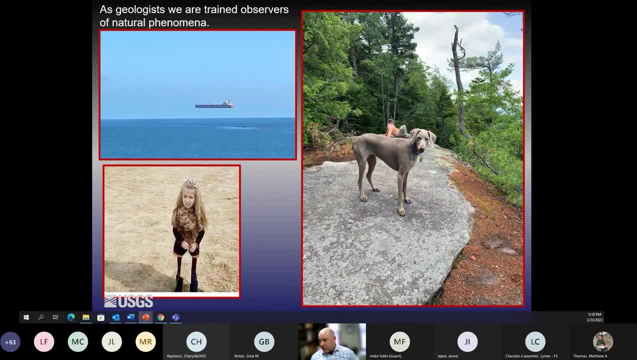 it doesn't really matter what we're studying. we face similar problems, since i've got sort of three slides here to sort of pick up where i left off again that i i found interesting and have incorporated here, because they sort of pick up with whatever we're doing, whether it's mapping or trying to figure out. 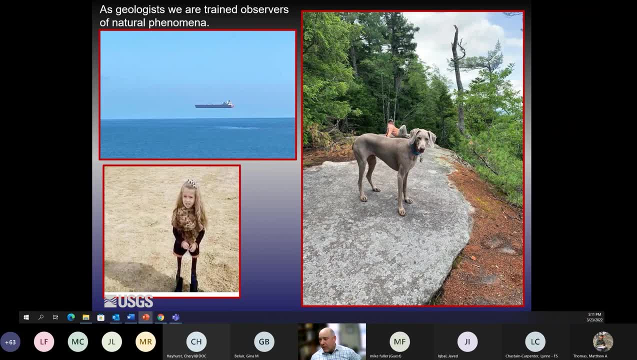 uh, landslides or groundwater, we never sort of have all the complete information, and so we rely upon things like interpretation. uh, we rely upon things, and this one here is in a mirage that was happened off the england last summer, which is kind of fascinating. uh, we, we see images. 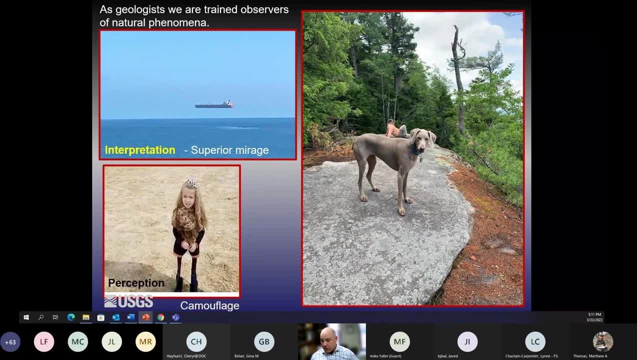 and we have a perception immediately. um, in this case, my first perception was that there's this: this young lady in the photo perhaps had a disability or had prosthetic legs, but in fact she's holding a bag of popcorn that is the same exact color as the background, grass, and so on, and 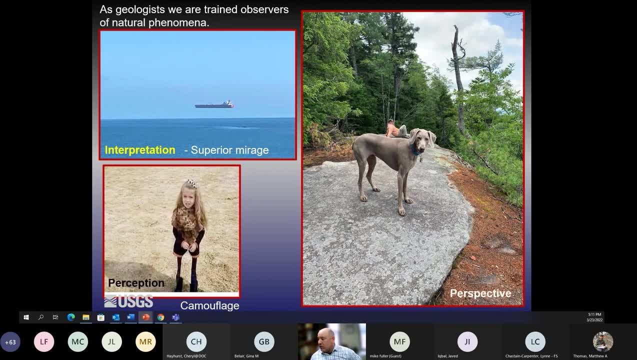 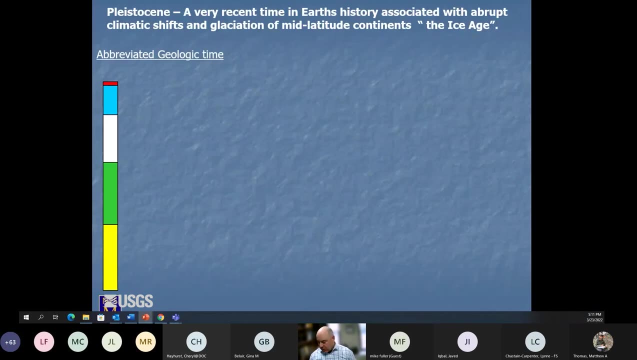 so forth. so it's playing tricks with our mind, and the other one that we're constantly dealing with is the issues of perspective and scale. so that is my dog, but that dog is not that big, um, so as we speak here again, all right. so again, i gave you fair warning. i'm a pleistocene quaternary geologist. so just to be thorough and 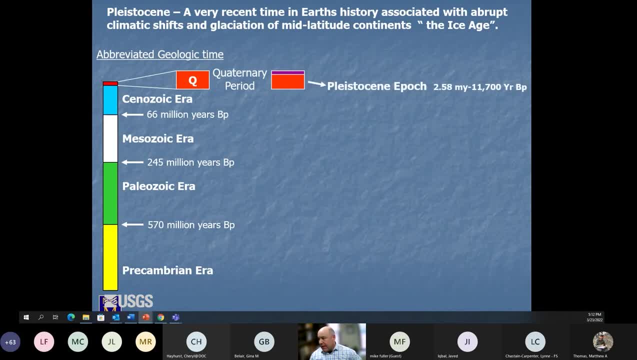 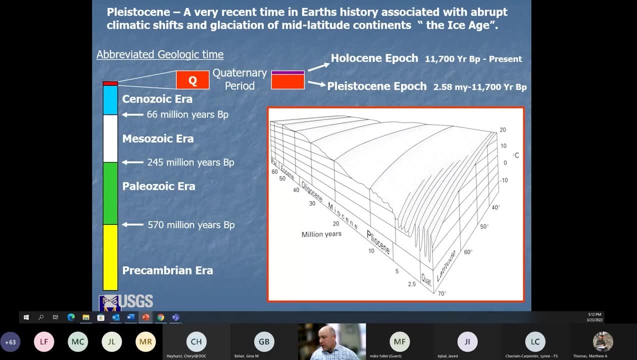 cover the sort of aspects of that. the place in epic, uh again about uh, 50 million years ago. climate starts cooling and then about the last five million to six, 2.6 million years ago, the climate really gets wonky and we go into these ice house greenhouse conditions across most of. 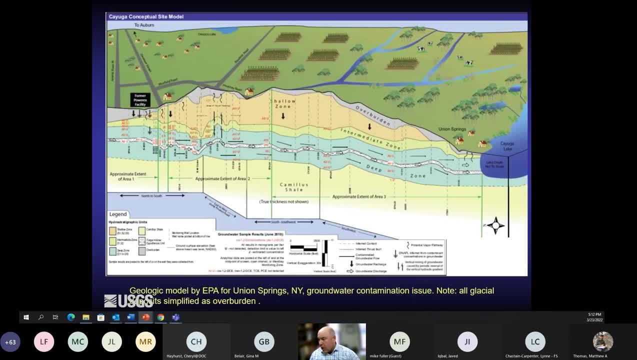 the northern latitudes, um, something that's been very common in new york state. in many places is is oversimplified, and so here's an example of a conceptual groundwater model, and all of the glacial deposits have been characterized as either drift or overburden, so this is one of my favorite. 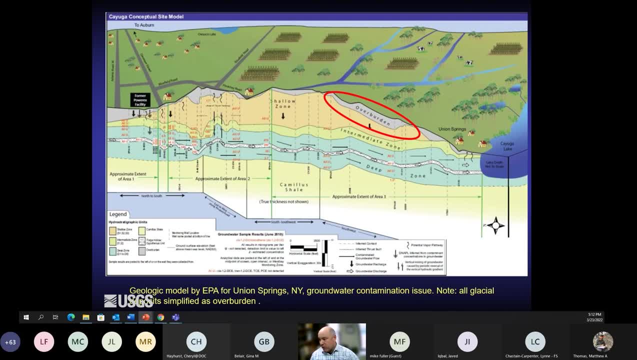 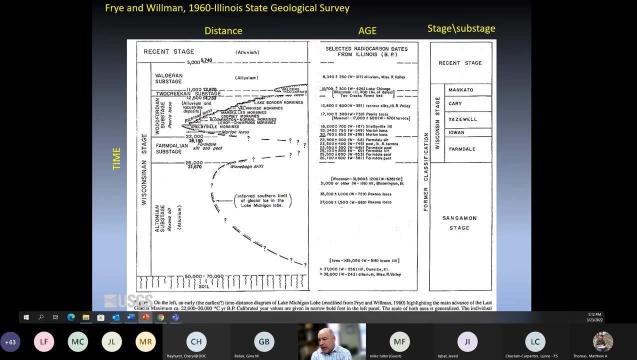 pictures, um, from an apa model. uh, just sort of showing us this oversimplification of it. and again, other states are further ahead than than us in many places in other states. for example, uh, here's a diagram from 1960 from the illinois state geologic survey, um, again, radiocarbon dating. 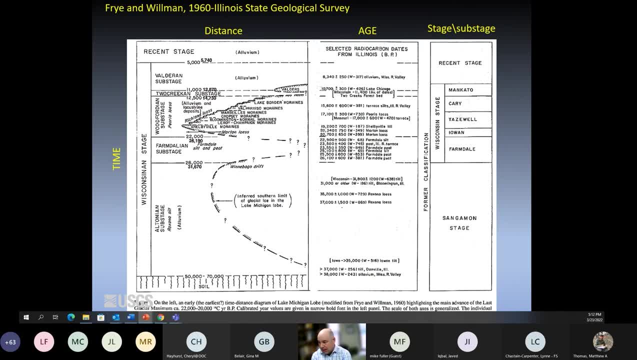 just barely been out, but this is what is known as a time and distance diagram, where they were trying to understand these pleistocene glaciations, understand the extent and the aerial extent of where glaciers were and their chronology and their timing, and establish their overall stratigraphy. 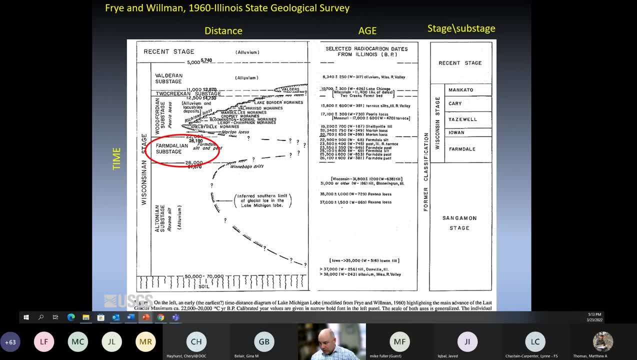 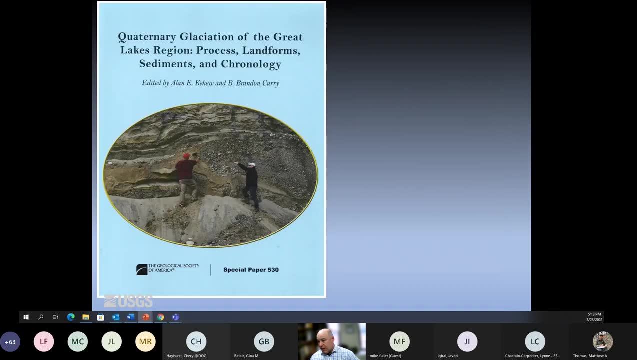 they identified certain important stages that were then recognized by other states throughout the midwest. but one of the problems we still have is that the geology stops a lot of times at the state boundaries. so what, what? what systems have been established in one state doesn't necessarily correlate to other states that have been done. 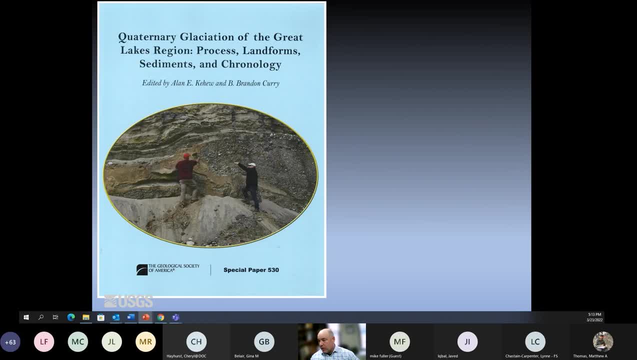 so some events. our work has been done more recently to try and correct or move forward with some of that. this is a recent publication from gsa on returner glaciations. uh, it's got some several articles in it, but here is a again on a modern, updated article from the illinois. 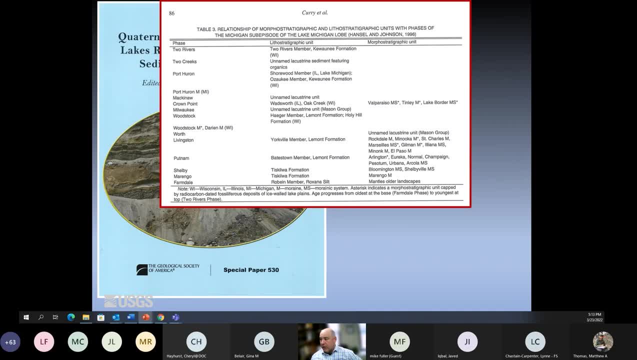 geological survey where, again they've gone as far as they have. they have lithostatic control, they have members and formations of their pleistocene units that they've worked for, and they've been able to develop time and distance diagrams that are more modern, with a better 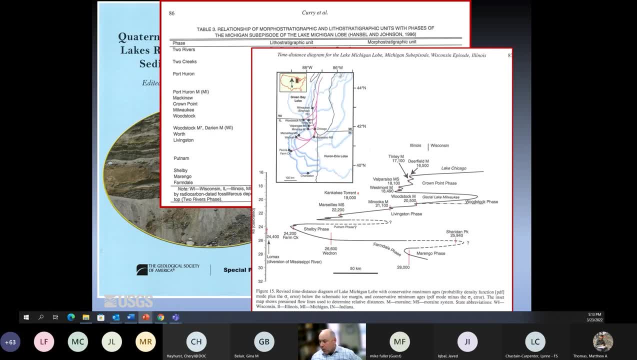 understanding about the extent of past ice sheets, and that's important because a lot of these past ice sheets are affiliated with large proglacial lakes and bodies of water and drainage, which ultimately result in lots of fine-grained sediments that can end up being problematic. 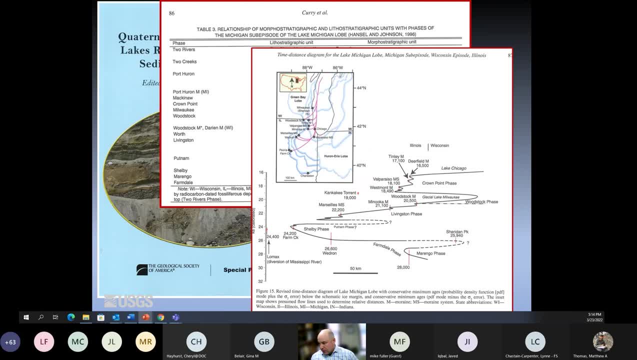 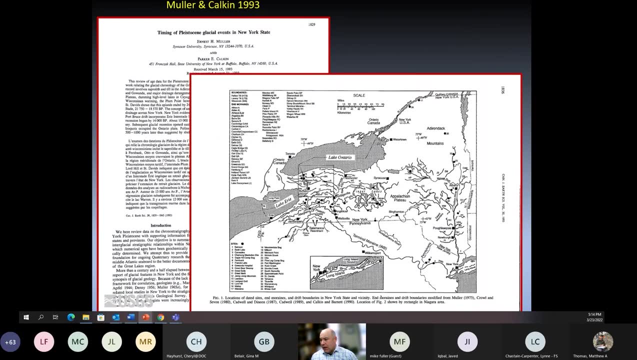 for slope failures as society builds over those materials here in new york, uh, one of the last real examples of this is the mapping diagram from 1903 by uh ernie muller and parker calkin, and it was based largely off of radiocarbon dates from the 70s and the 80s to sort of establish control. 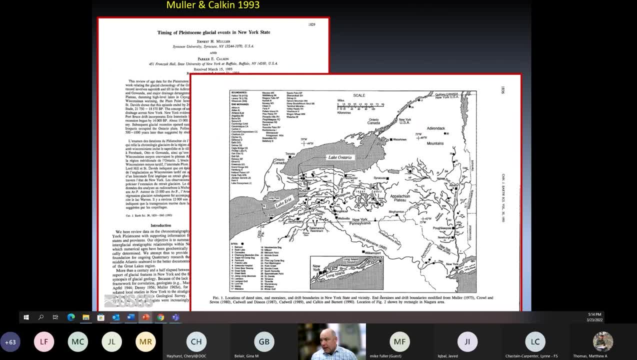 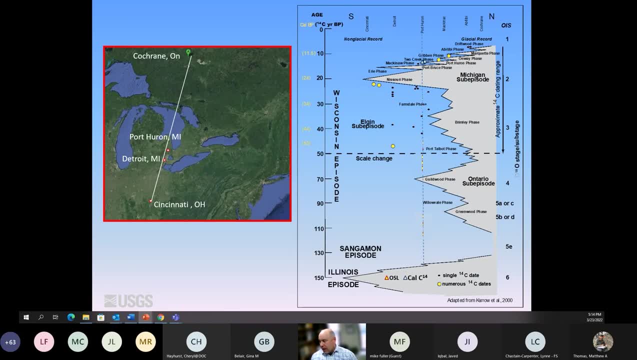 um, and that's sort of the limit of what's been done largely for new york state, um elsewhere in the region. this is a diagram again from paul carrow out of canada and it's a time and distance diagram showing again from cochrane, ontario, to cincinnati at ohio. these uh sort of spikes to the. 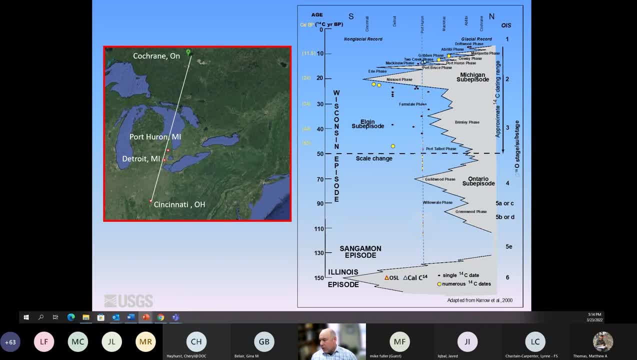 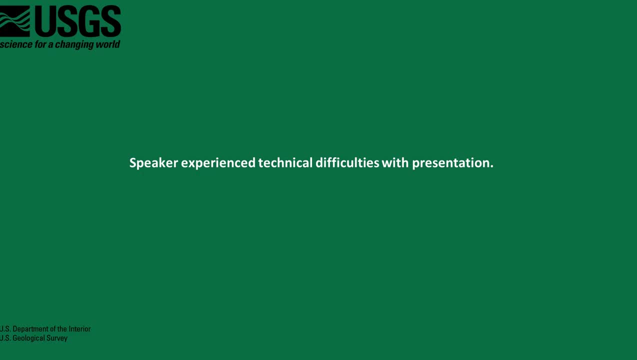 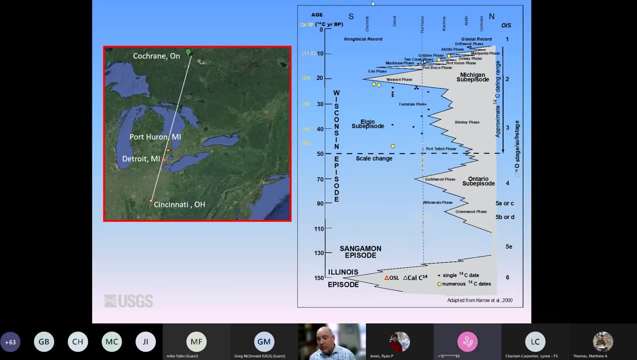 screen are sort of further to the south and they've got radiocarbon control and they've got they're showing the oxygen isotopes, all right. so anyway, the point of my slides, before i bailed on all of you folks, and i apologize. we don't have an understanding of chronology, we don't have an understanding of stratigraphy in 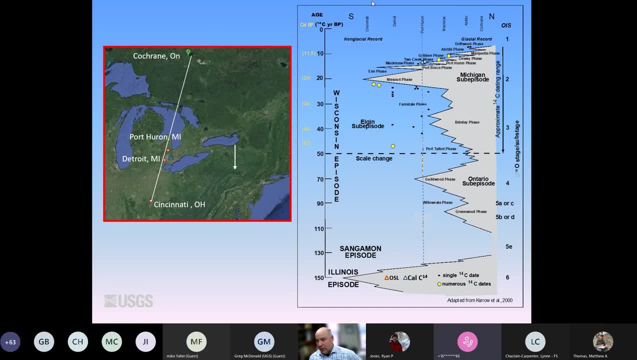 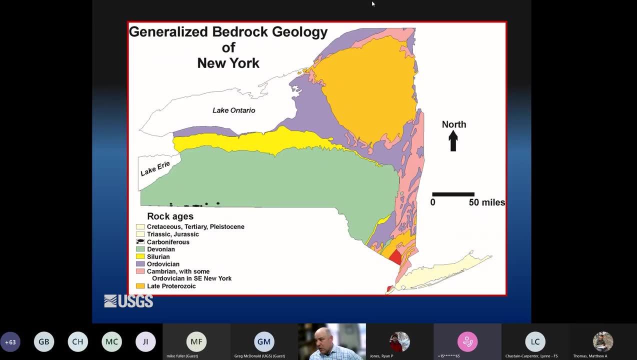 new york state, um, and that's what we've been working on. that's why we've been mapping where we have been mapping. um again, continued overview of our state with a bedrock- uh, slight dipping paleozoic rocks throughout much of the state, but it has a big impact on our places in glaciation. 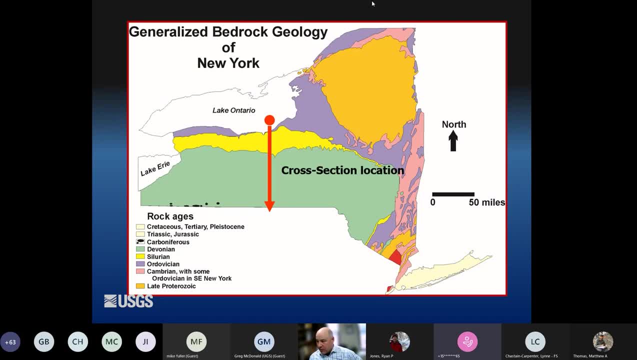 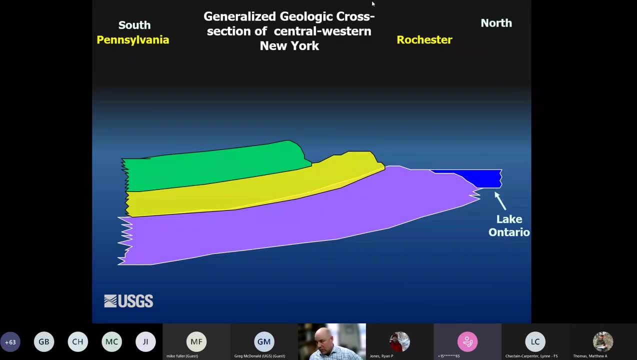 so if we looked at a cross section across new york state, from ontario to pennsylvania, we'd see that the rocks are largely dipping slightly to the- mostly the south- and slightly to the west um across the plateau. again we have lots of these limestone escarpments across new 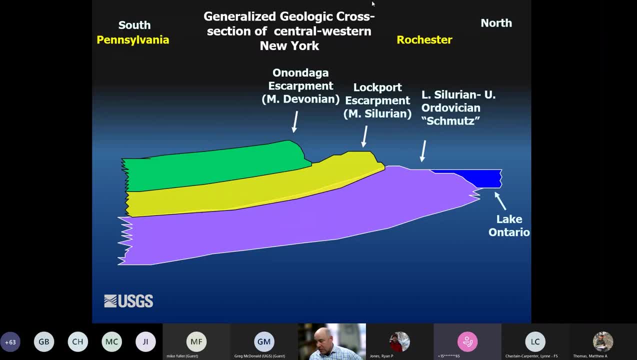 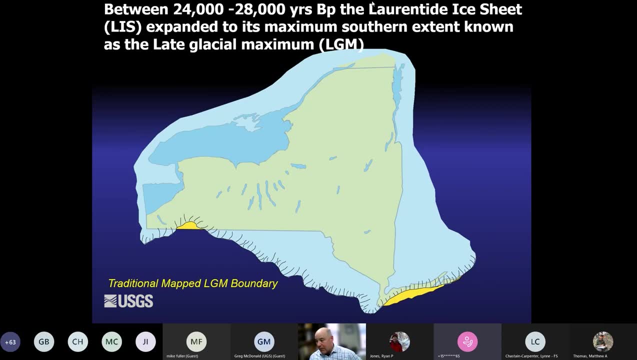 york state and the end result of this is that basically again has impacts with overall deglaciation. so overview of glaciation: according to our trip, typical mapping of what we have is that during the late glacial maximum again all of the states covered with ice, except for a small part of western new york, southern long island, um the laurentide ice. 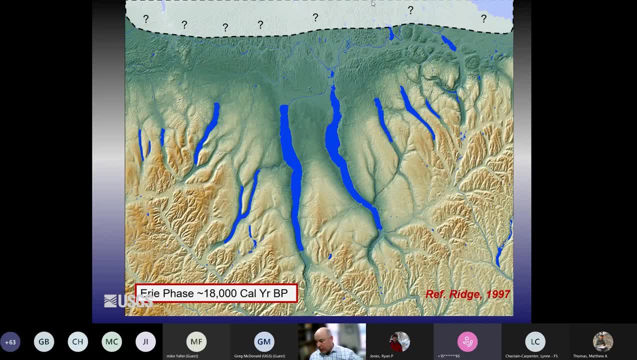 sheet sort of rifle. through these try and get caught up a little bit. there's a period of time known as the erie phase, which where the ice deglaciates out of the finger lakes region completely and restores drainage to the mohawk river valley. 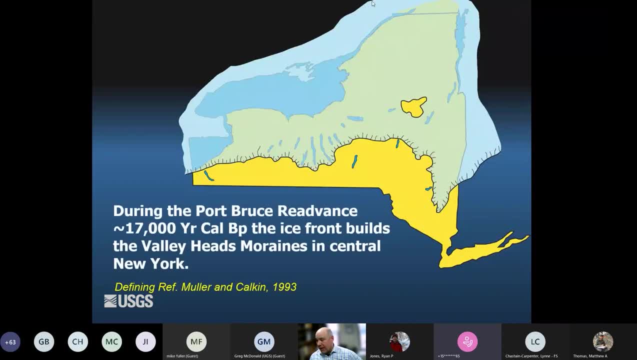 the ice re-advances at this stage, known as the port bruce, or forming the valley heads moraines, which is important because it creates the modern drainage divides between the ontario basin and the susquehanna river drainage systems into pennsylvania. so the ice is re-advancing during this period of. 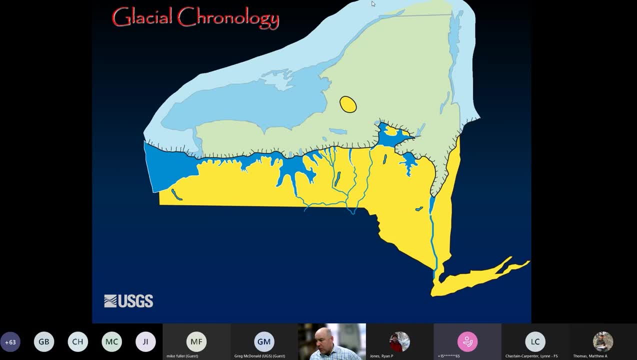 time and then, of course, as it retreats back off of those bedrock escarpments and it's carved out, it creates these small, sea-sized pro-glacial lakes. very large pro-glacial lake systems trapped between previous bedrock topography and new, new areas have been carved out by the glaciers. these 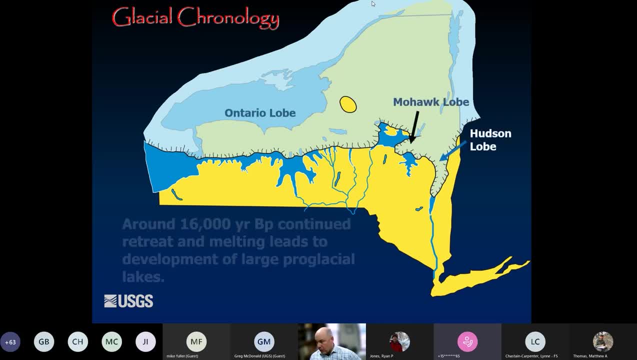 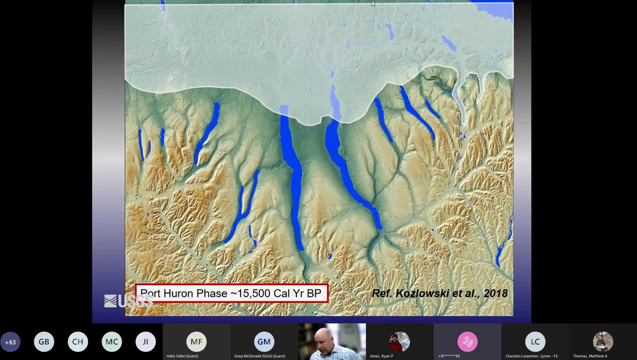 glacial lake basins, and so again, the various different lobes across new york state are establishing a multitude of pro-glacial lake systems across the landscape. and again, lastly, there's oscillations of ice advancing back and forth. this is a sort of an estimated chronology. 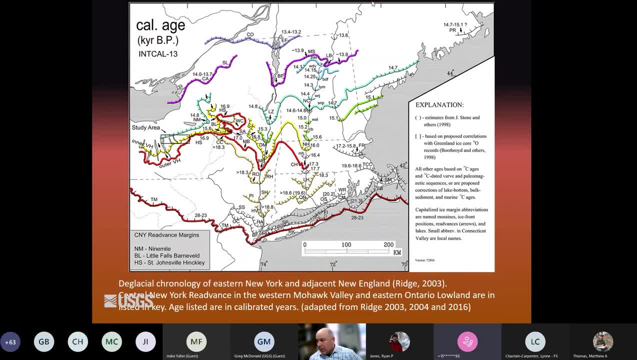 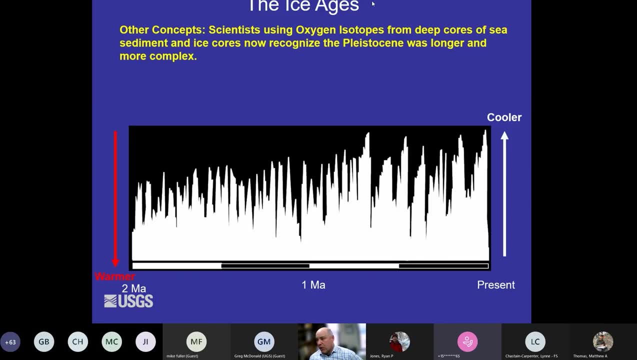 coming out of new england based on the new england barb chronology. um, and so another point to all these slides i've been showing you about chronology and saying we don't have them we do have is that none of them match up with a larger scale global record of ice ages, such as those: 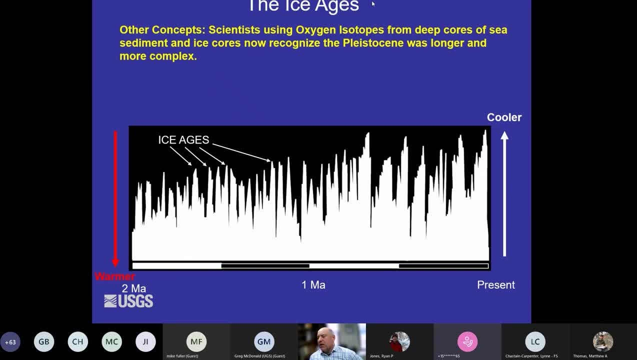 recognized by deep sea cores and, in the um, ice cores from greenland, so on and so forth. so again, we now recognize that we still think there's only four or five glaciations, but we realize that there's this oscillation in the last 2.6 million years, right, and we've got all these glaciations. 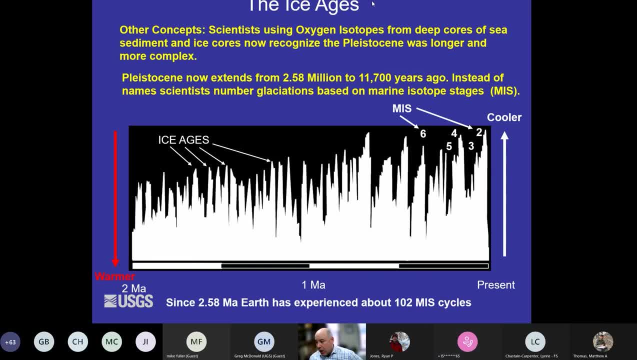 and conditions possible for glaciation, including about 102 of these mis marine isotope cycles across the northern latitudes. but we don't know or recognize individually often the sedimentary packages left left or preserved or available still to be engaging with uh societies we build over. 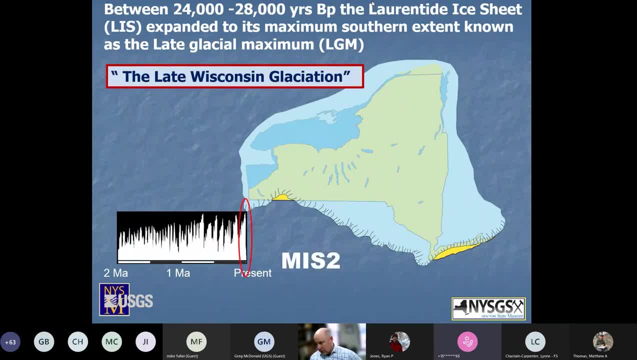 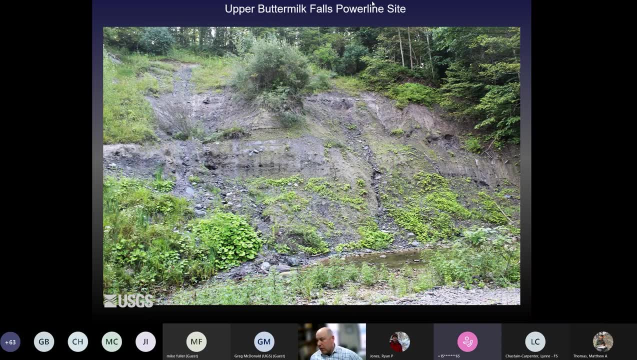 these deposits, and so the last, most recent one of these is mis2. um, all right onto some geology photos. so these are typically what a lot of our upstate new york outcrops look like, and this is along streams where we have a lot of our slope failures. um, we have a lot of our slope failures. 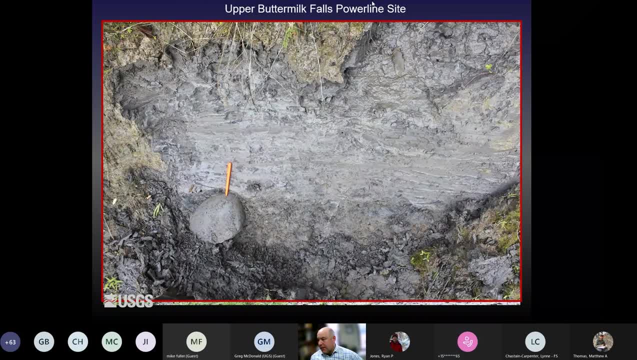 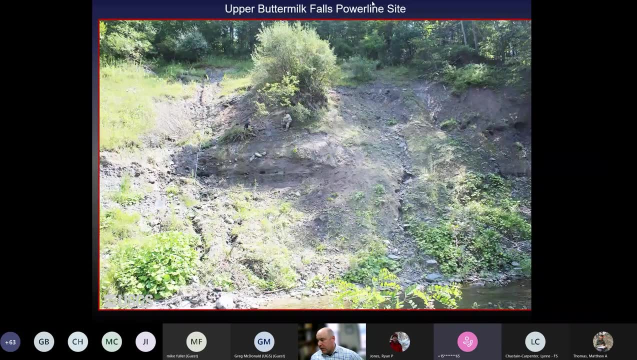 and we have lots of laminated lake sediments. they're often interbedded with other deposits um showing sort of field photos. having to rifle through these are going to get caught up um again for scale and and in these photos we've got again multiple glacial till units, multiple. 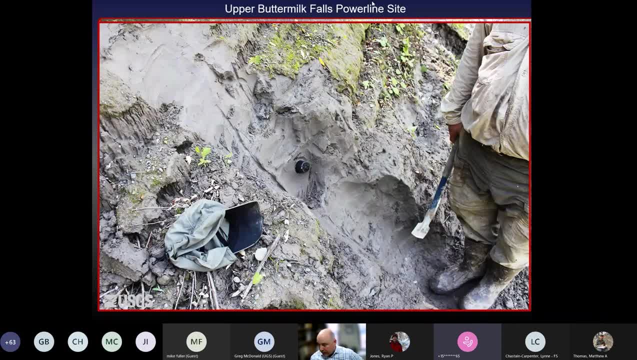 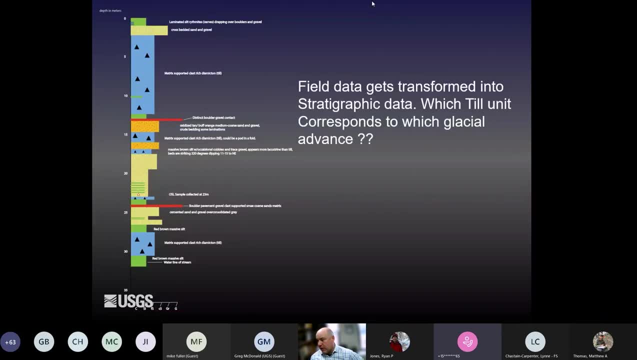 lacustrine units, silts. here we are collecting a sample for our optically stimulated luminescence dating, trying to get a handle on chronology, um, and so here's basically right. we take our field data, we transform it into this and then, of course, we have all these blue colors. 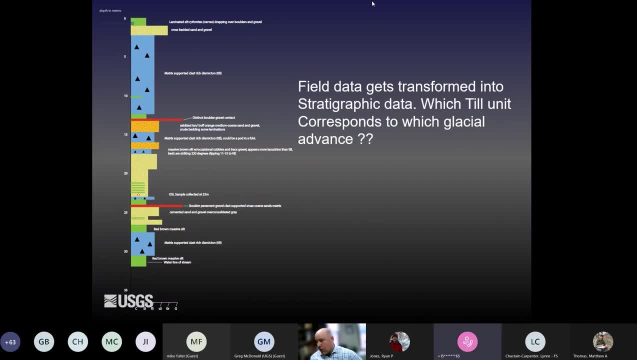 which represent glacial till units and, as i've just dazzled you with all of this chronology and this oscillation of ice fronts, which glacial till unit corresponds to which glaciation? and this is part of our three-dimensional puzzler game we're playing here in new york and other. 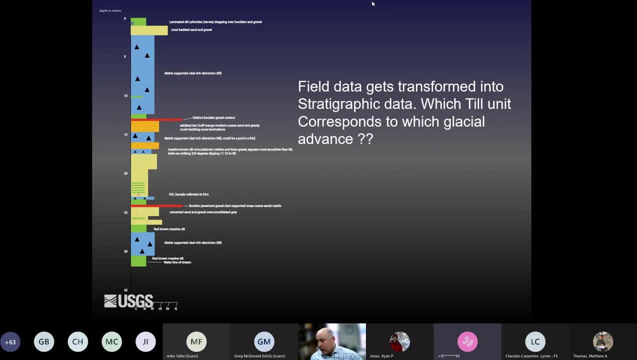 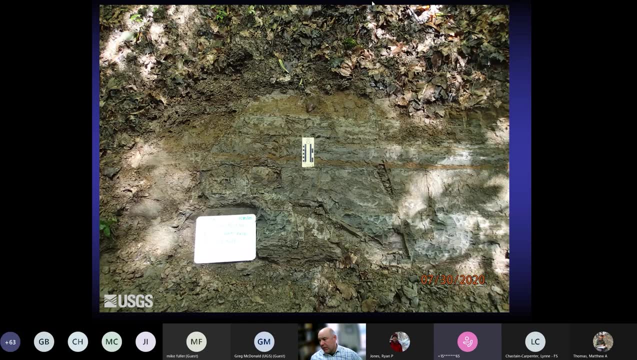 places in new england as we try to understand the 3d framework of these glacial deposits, and just as another example of this, here's a photo of some some really indurated tough lacustrine sediments. these lacustrine sediments have actually been faulted. there are a couple of 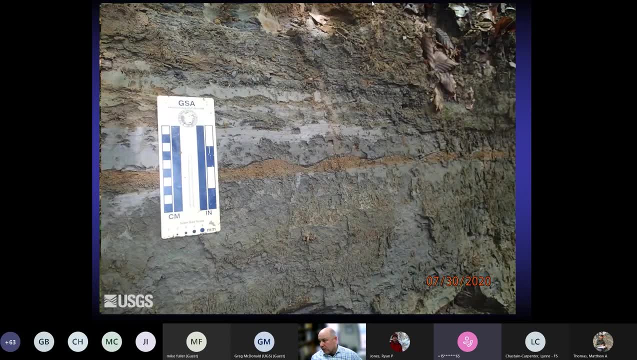 uh locations, but they also preserve some fantastic structures, such as some very nice ripples, so on and so forth. so this is typical from the outcrops we would see and work on, except that in this particular case, in these ripples, we've recovered arctic. 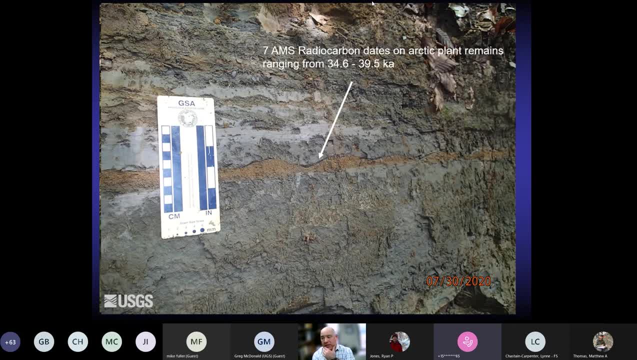 plant remains of arctic tundra, dryas and salix leaves, which are basically about almost between 35 and 40 000 years old, which tells us that this lake sequence is actually from mis3, or it's a lake sequence that was established before our most recent glaciation. so understanding chronology is. 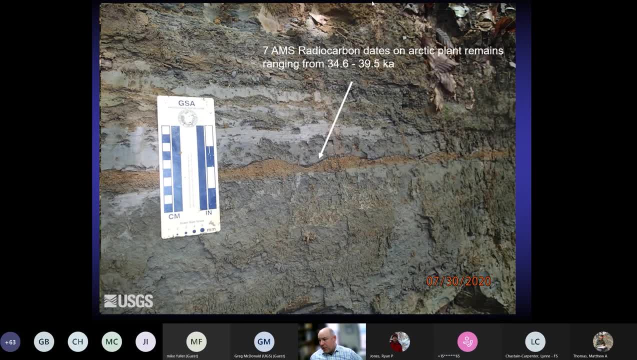 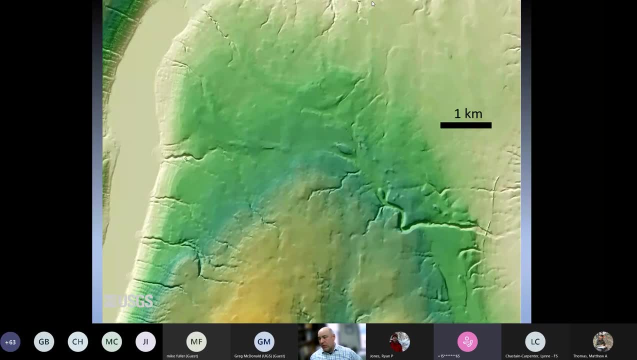 really important for our framework as we move forward with our mapping. the other thing that's been really helpful as we're going forward, like it has been in all states, is the advent of lidar. so here's the lidar image that we would have used. i would have used in graduate school in the late 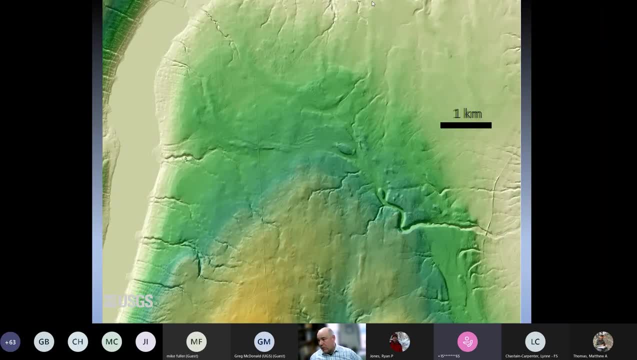 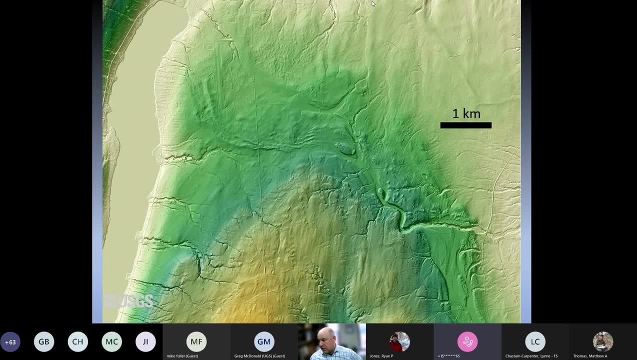 90s and that was a 10 meter dem you're looking at. and now, of course, we have one and three meter scale, lighter images that show us moraines and all kinds of humic topography and spillways and streamline landforms. so mile is taken out of theıp and it actually takes our job a lot easier than it used to be. 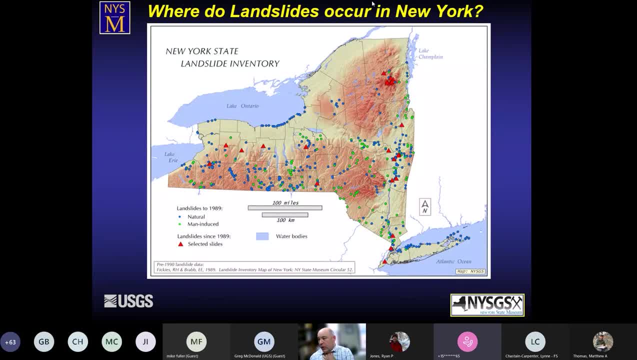 landslides in new york. where do they occur? everywhere, but there's a couple of key locations where they've occurred with greater prominence, greater prevalence, and that is the hudson valley location in the adirondacks, which is what i'll focus on. with these next couple of locations, we're 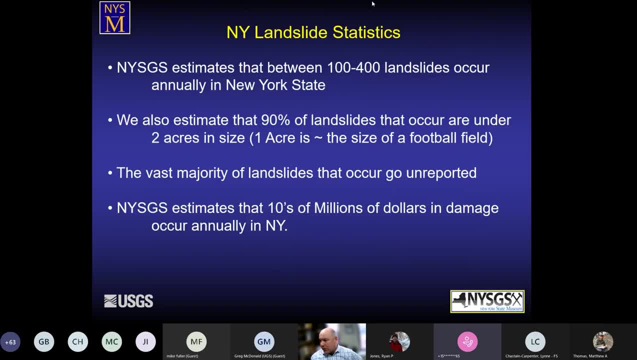 working through in these slides? um, we estimate that there's about 100 to 400 landslides annually in new york state. most of them are extremely small, um, typically under two acres. they almost all go on because, unless they're affecting a road. that's when our Department of 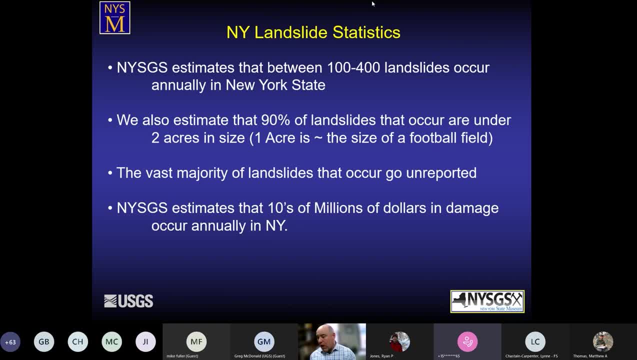 Transportation would get involved and call us or let us know they're on private property. we're not regulated, we're prohibited from working on private property. so again, a lot of these go unreported. but we know that they cause many tens of millions of dollars for the damage annually, whatever the process may. 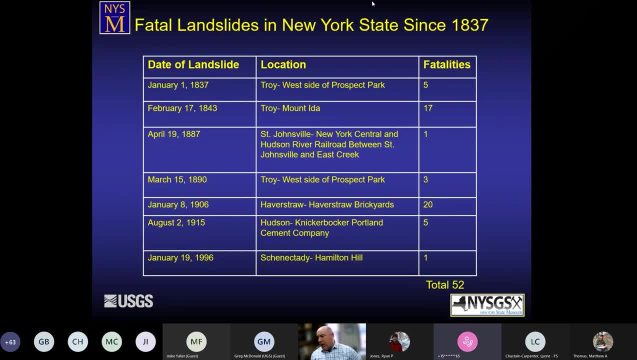 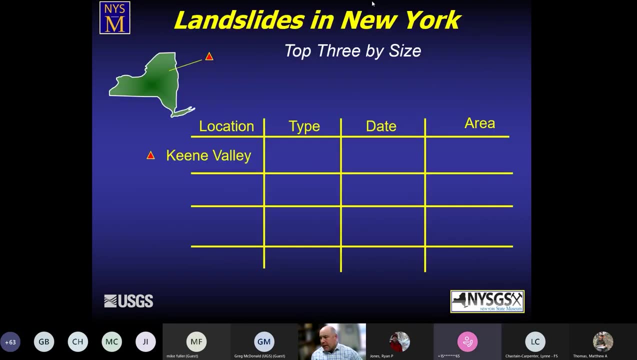 be, and again, some of these landslides in New York are fatal, so we had a total of 52 fatalities since they've been recorded again. most these locations are in the Hudson Valley and many locations. I'll circle back to some of these sites a little bit later in the talk. as I rifle through things, our landslides are: 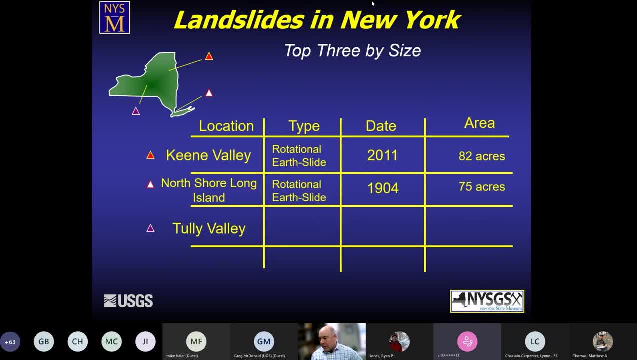 probably small compared to many states, especially out west, but these are the big three again: 82 acres, 75 acres and 53 acres. I'm going to spend some time talking about the Keene Valley slide and show you a couple of photos of this more recent slide from Tully Valley. 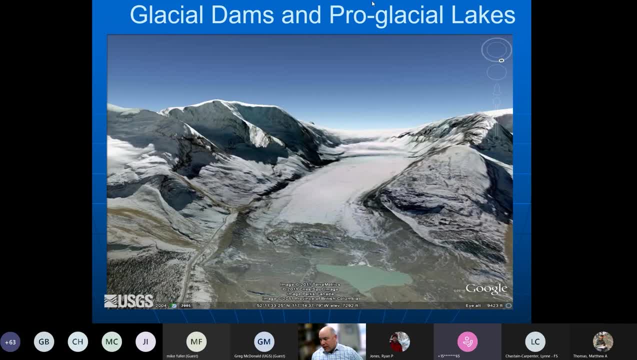 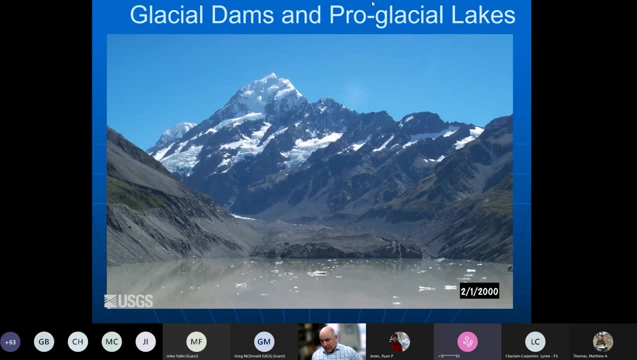 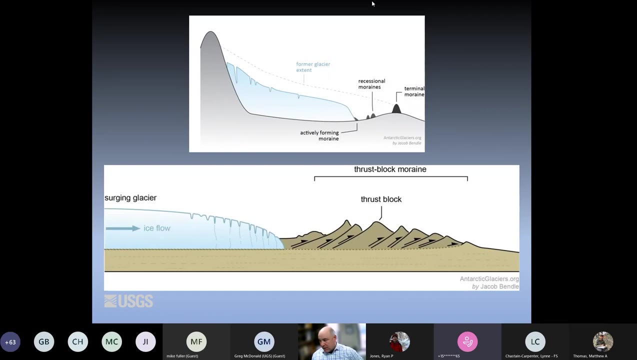 so again, as I've talked about before, with the glacial landscapes and these things, the problems we're facing here are again are associated with glaciers that are trapped in valley systems, again that they haven't formed proglacial lakes, so again ice is advancing down, build a series of different moraines. 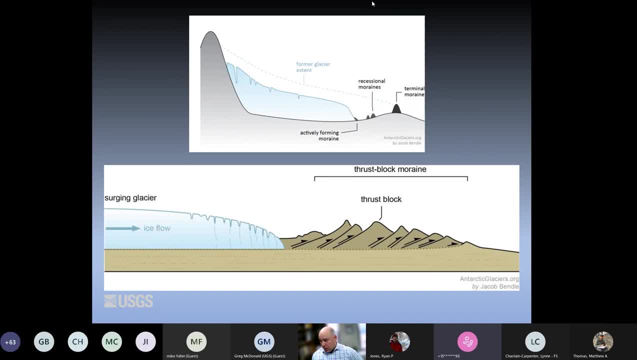 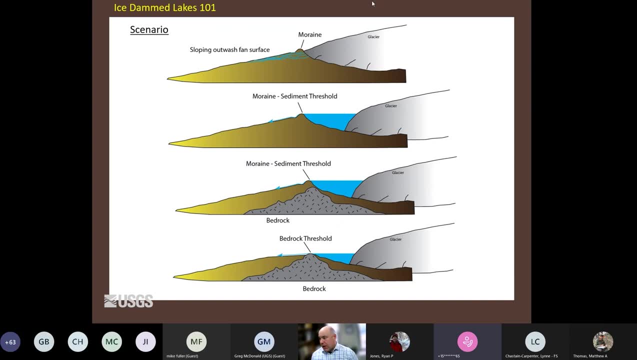 sometimes small-scale recessional, sometimes large-scale thrust block or sort of large-scale moraine systems, and then, when the ice is pulling back out, where the ice is pulling back out, we have the possibility of creating these moraine: sediment threshold, controlled ice trapped lakes or if they erode through. 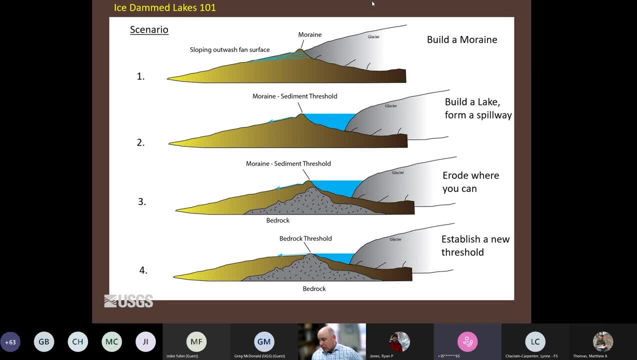 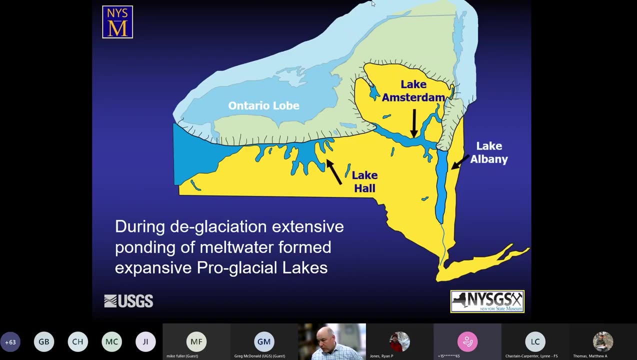 basically a series of sediment. they may encounter a bedrock threshold and then ultimately, if the ice retreats far enough, it will simply find new outlets. but we have the ability to put a lot of fine-grained sediment high on the landscape as a result of this, and that's sort of important overall. so again, here's. 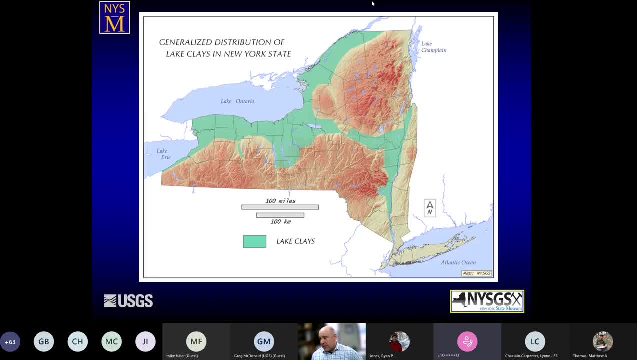 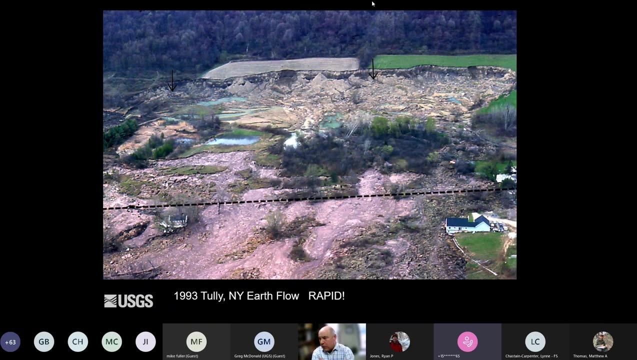 sort of this overall footage of of the� or the clays and the length of the lakes, and the net result is that we have lots of lake clay spread out across New York State. this is a very generalized map, so on and so forth. this is the 1993 tully landslide, which is classified as 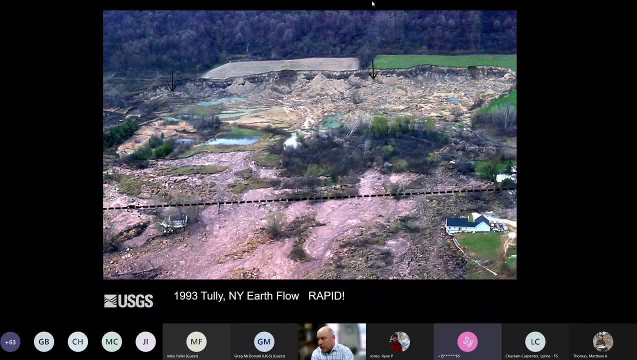 an earth flow, a rapid earth flow system. the dashed line in the photograph you're looking at is a road. it's completely buried. there's a house over, sort of on this portion of the screen here. this house was located on the other side of the road before the next 10 or more years and it was another angry. 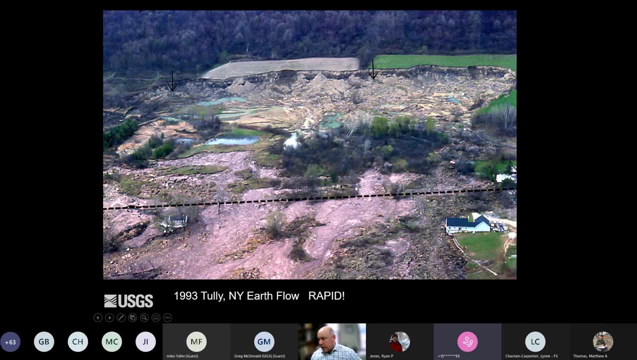 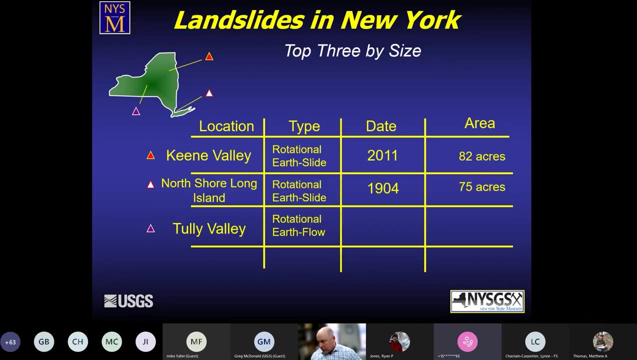 landslide happened. no fatalities occurred with this landslide, but a lot of displaced houses and in quite the mess taking place. again, these were in glacial lacustrine clays and some of these steep wall valleys, uh, throughout the finger lakes area of central new york state and again sort of 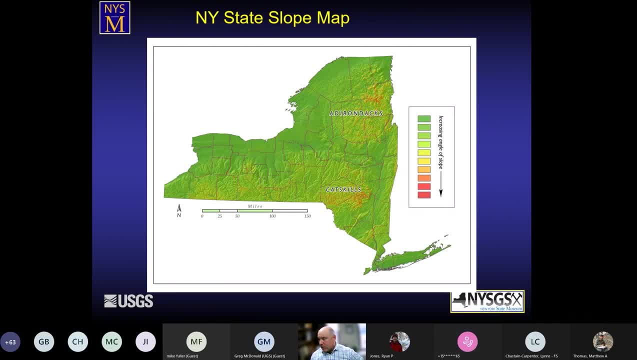 going back through, moving into sort of the adirondacks and that area. so this is a general map of the slope of new york state, and the highest or steepest slopes in new york state occur in the adirondack mountains and in the catskill mountains. um, and so we zoom back into this next story, which 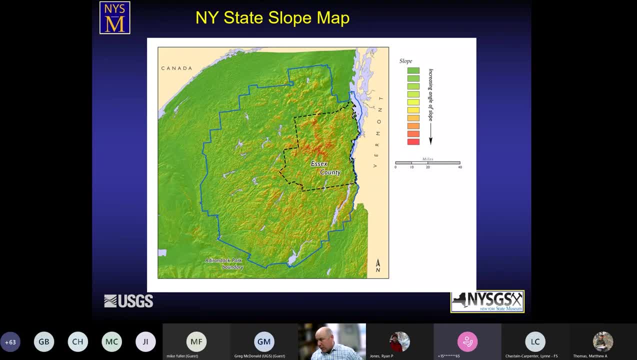 is related to a slide that was a little bit same as about 10 years ago in the adirondacks. so a couple of things. the adirondack park is something that's talked about a lot here in new york state. um it and it's confusing because it's, it's just, it's not a, it's not at all public land. 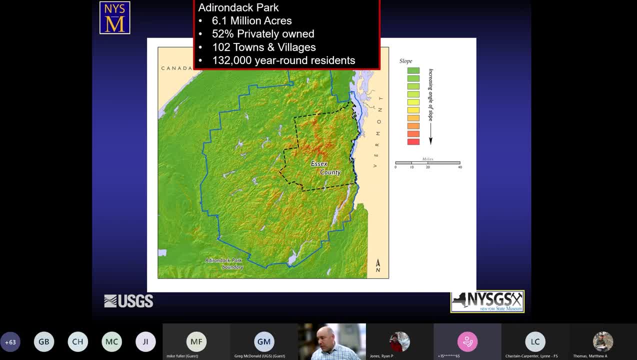 all right. so it's about a six million acre area. uh, half of it's privately owned. there's lots of villages and towns and it's kind of a little bit of a different landscape than the adirondack mountains. so it's a little bit of a different landscape than the adirondack mountains. 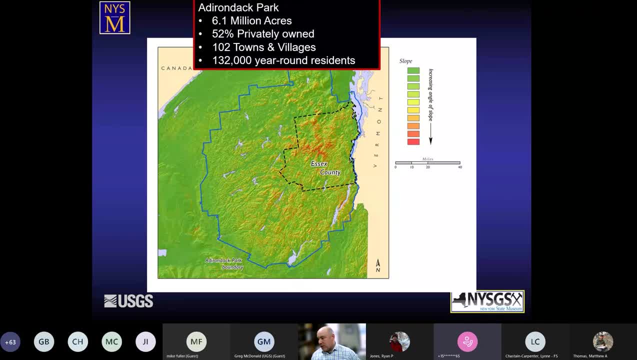 a very sort of low round or year-round population. uh, given the size and scope of the area, that uh that it, that it contains regulation and permitting in this area is- is controlled by a governmental authority. it's administered by the, by the governor's office. so the governor's sort. 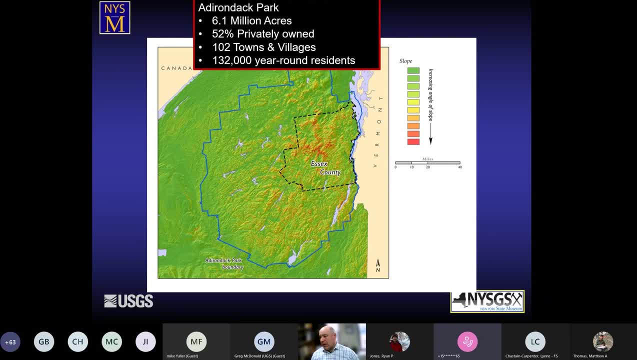 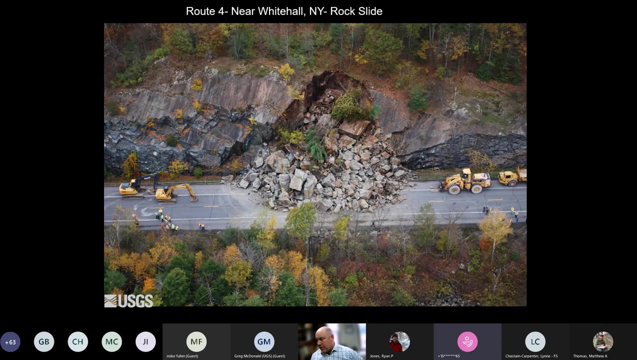 of uh authority often can supersede whatever regulations and permits are issued by towns and villages, which leads to all kinds of happy, warm, fuzzy feelings, sometimes by residents in these small towns. so this is just a sort of again, my talk is focused on glacial place to scene slides, but this is a typical slide we would see somewhere in the northern adirondacks. 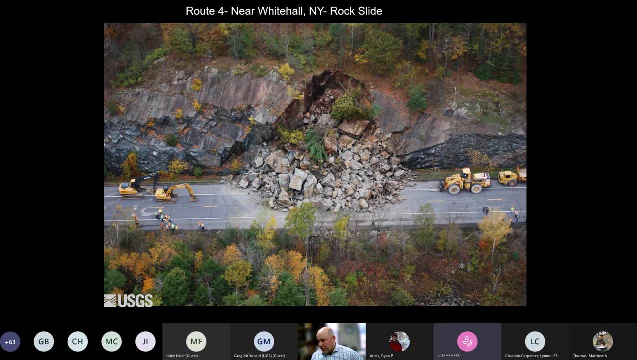 are rock slides again. this is near whitehall and in sort of the eastern edge of the adirondack mountains, uh, showing a typical road blockage, um, from sort of rocks that are sort of dipping or jointed, facing the road systems again and again. smaller scale compared to 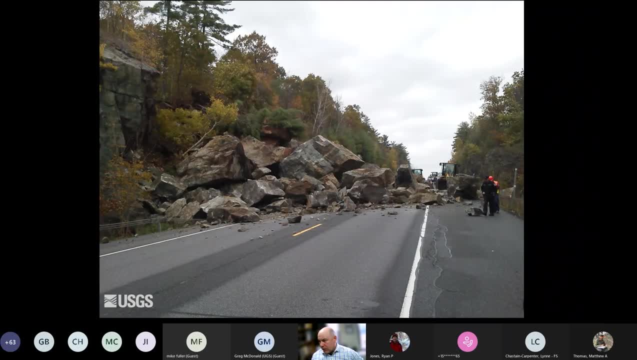 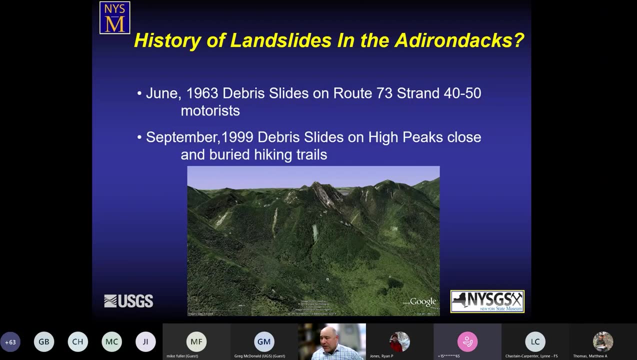 probably many slides out west or elsewhere, but a pretty good size rock slide for here in the adirondack mountains, new york state. um landslides in the adirondacks. there's a fair history of these things. the vast majority of landslide events that occur in new york state in the adirondacks. 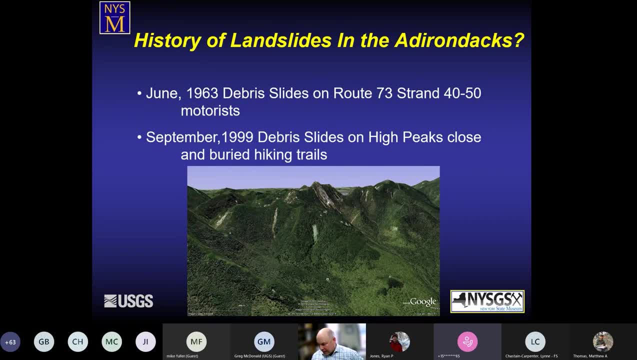 are related to these debris slides or debris avalanche type slides that occur. they're almost always associated with tropical storms or hurricanes. um, you can see scars. this is a sort of a google earth image of a giant mountain in the adirondacks and you can see. 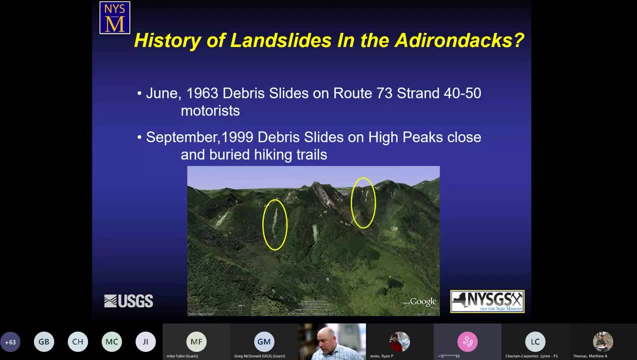 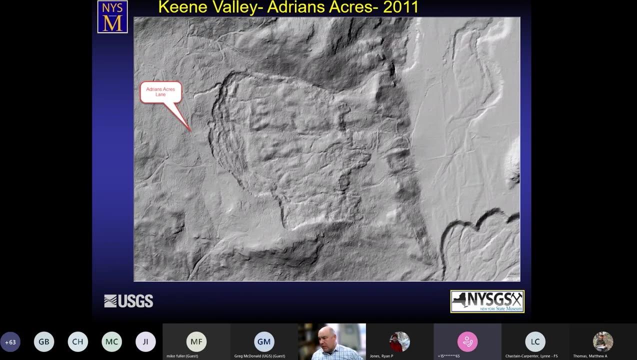 these landslides. from the avalanche, debris flows there on the mountainside again very quick, very rapid events. when the soils get saturated and loosen, all the trees and rock comes down on the landscape. however, in 2011, we had a completely different beast that developed, known as the keen valley landslide, or sometimes referred to as the adrian acres landslide. this 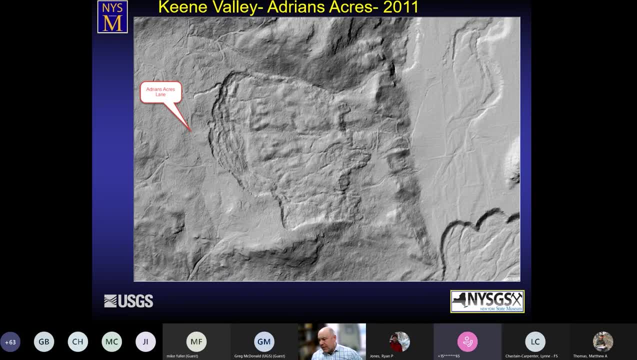 is the largest landslide in new york state history, about 82 acres in size, um, and it was right up on the in the high peaks, some of the highest slopes within the adirondacks- there's a bedrock ridge at the bottom of this illustration. you can see the road systems from. 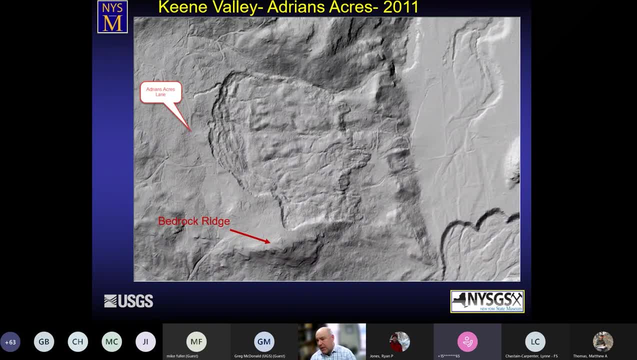 where they're housing as it's been developed. one of the things that's happened in the adirondacks- that's like other places- is that the the number one go-to destination is lakefront property. but as the lakefront property gets purchased and taken out of the market, the next place is places with a. 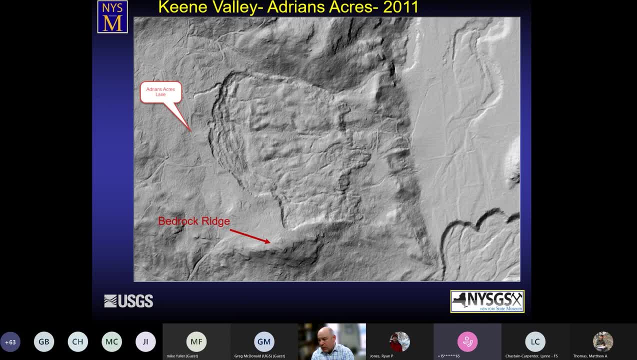 view, and so when you have lots of high mountains and steep slopes, you can get some spectacular views, which has led to development on these steep slopes which is largely unregulated in new york state. so this is the, again a footprint of the keen valley landslide. again, it's not. 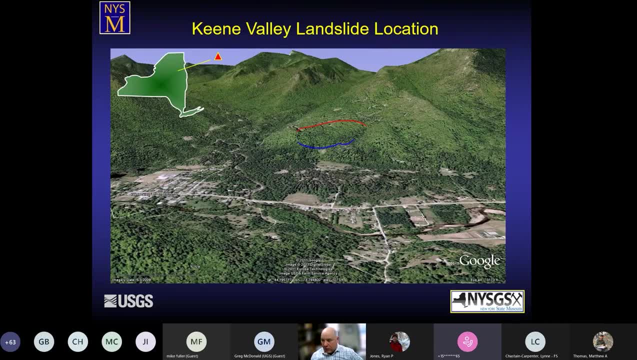 necessarily the steepest part. it was activated around uh sort of may 1st of 2011. we received some phone calls that there was some slopes, uh had moved, some houses had maybe shifted, and so we went up into this region to sort of look at this again. and red is the. 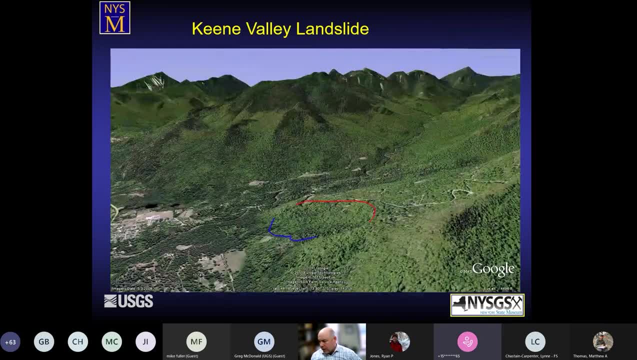 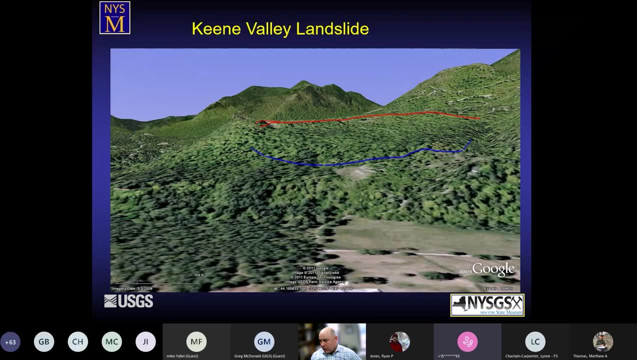 headscarp and the bottom is the toe and blue just a couple of other angles to sort of show. it's again relatively not as steep as other parts on the landscape that you might see. um, all in all in general, this was sort of uh occurred, or again right around may 1st, we would say. 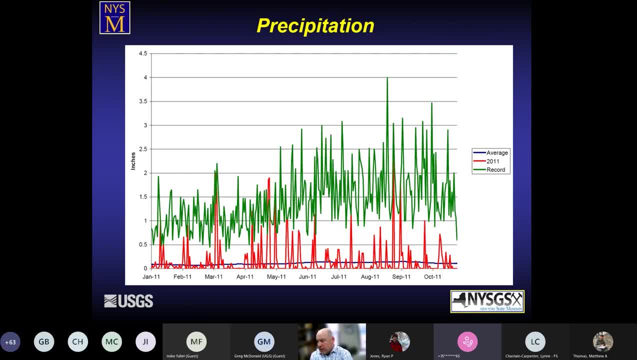 so there's a typical precipitation for this region that we would see again. you can see the, the average, the record and then, of course, the precipitation for 2011.. that particular winter we had a very high uh snowpack from some late winter storms, so we had some pretty good rain. 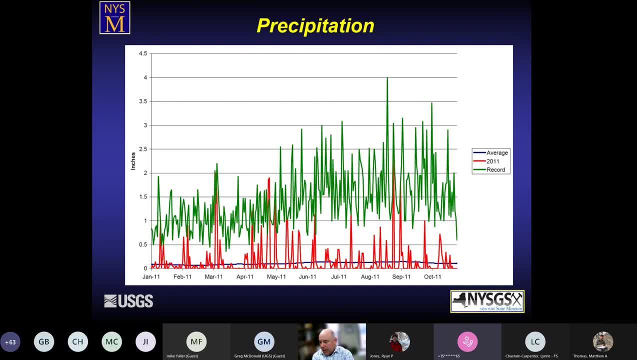 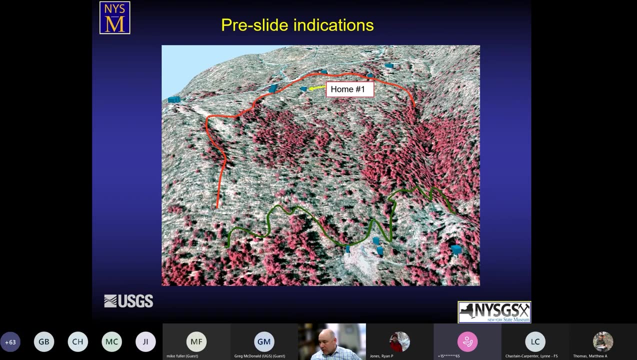 on snow events up in this area. that may have been part of the partial trigger for this landslide to um uh when we were looking at the area and working on it. so that's sort of the precipitation event. uh, as we dove in more into this, there was other sort of pre-slide indications as we began to. 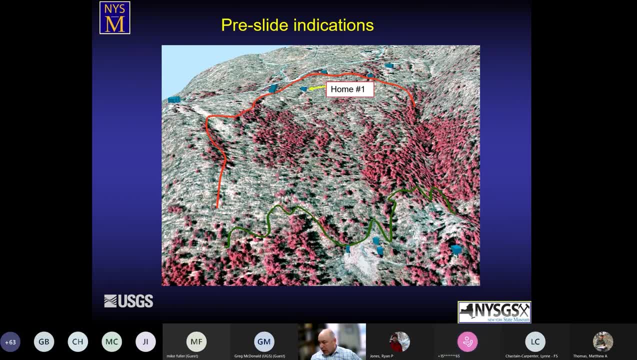 talk to people that home number one- you see in the screen- was destroyed. uh, home number two was damaged, i think ultimately abandoned as well, home number one. people began to report that their- uh, their windows and doors have been sticking for some time, right, kind of classic signs and uh, there's something that's going on. but they were just sort of seasonal homes. 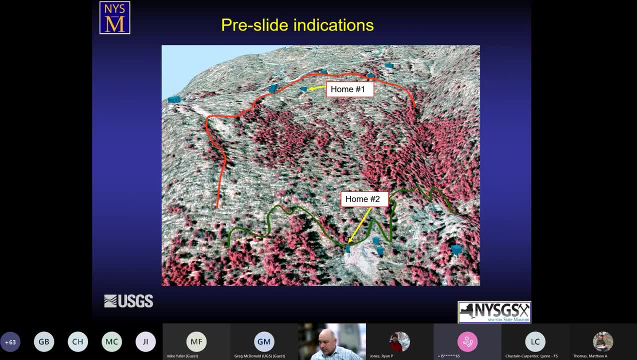 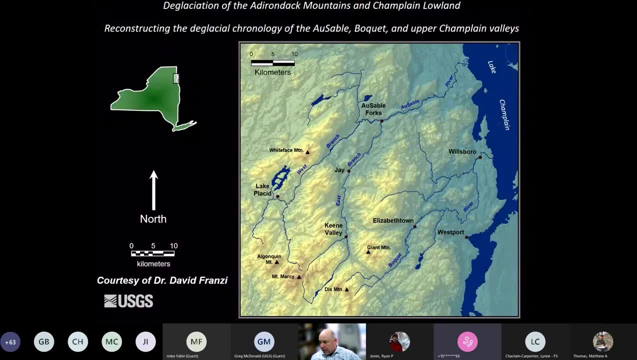 built. this home was built back in the 80s in this particular location, um and uh. so the context of the landscape- whether there's keen valley sort of located there, giant mountain- is another one we looking back to in a moment here, but just for reference. so we're at the, the intersection of 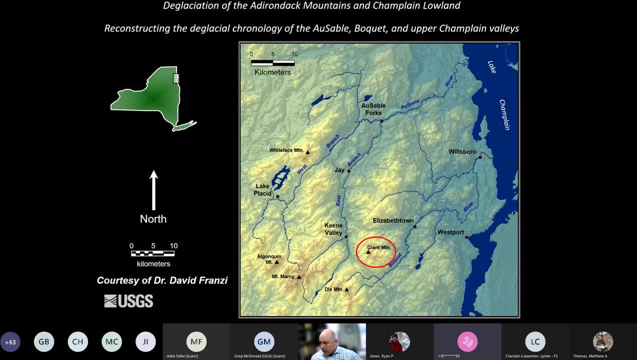 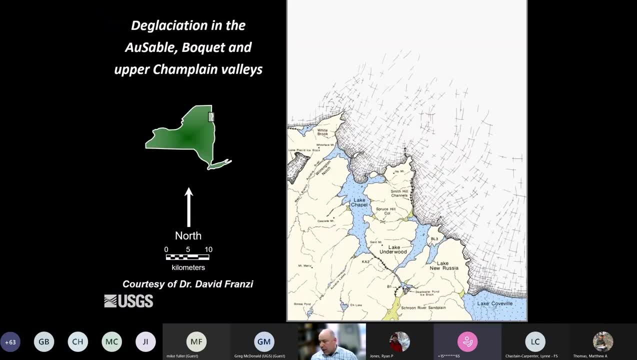 these branching streams, the east and the west branch of the osable river flowing into lake champlain. but during the ice age, the last deglaciation um this, these drainages were blocked. there's giant mountain again for reference, um, and so the keen valley area is right over here on the. 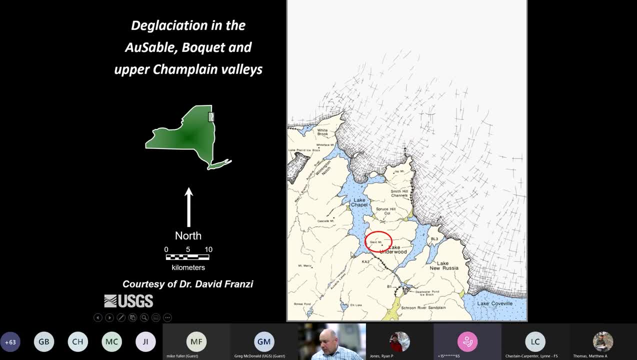 slides, uh, and and then uh, this large lake, lake chapel formed, which may have been as deep as 800 to a thousand feet in a couple of places. it was an exceptionally deep proglacial lake trapped up against the high peaks of the central adirondack mountains in this location. so here's just some. 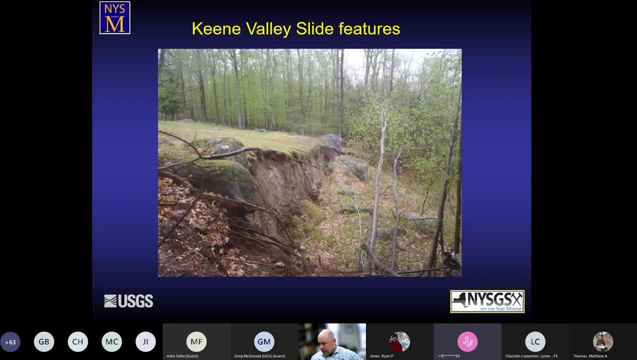 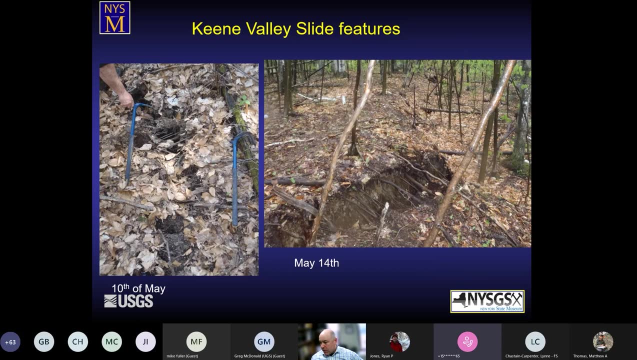 slide features related back to the landslide. again, the uh, the headscarp, the developed proglacial developed pretty soon after the slide itself triggered um again photos. it was really very active in the early parts of may and through uh through june, um again sort of typical uh spreading. 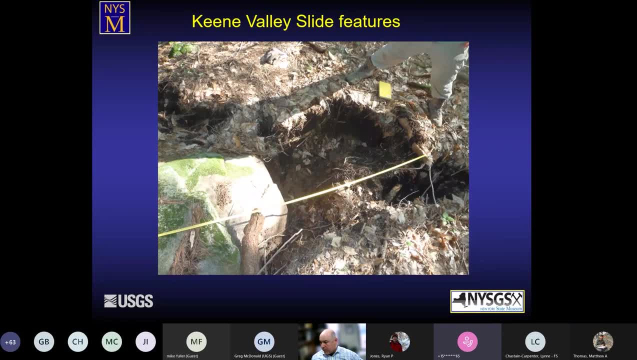 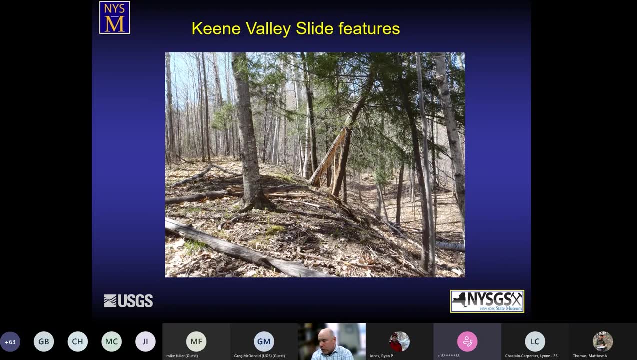 of uh these tension cracks the surface of the top the slide scale. this slide is interesting because it shows some of the trees that are splitting, where the trees grew and they in this particular slide. it's interesting because it's it's growing on the older headscarp. there was an older scarf at the top of the slide. feature: geomorphic expression, a couple. 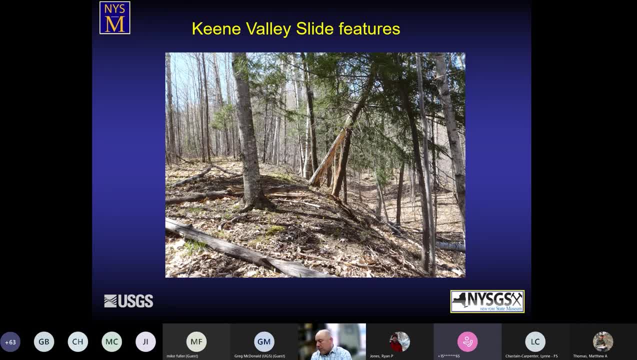 of the trees had fallen on some homes. when the trees were cut down, we counted 100 plus rings, so the trees had been stable on the scarf for at least 100 years. it had not moved. so in this case this was a sort of a very slow moving, or it doesn't reactivate that often so 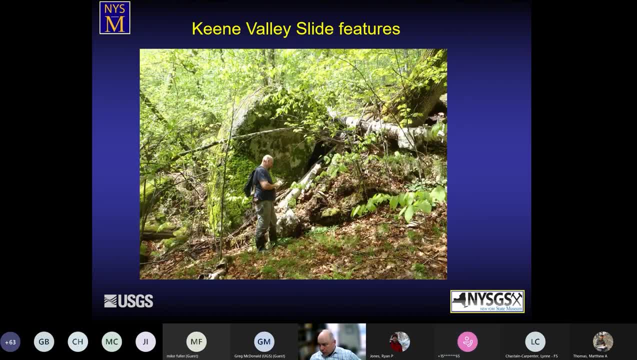 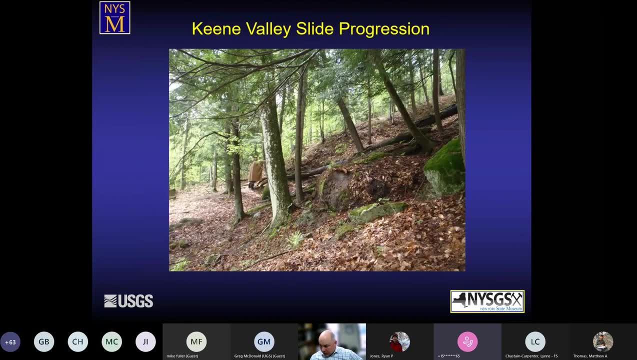 to speak for the size and scale of this particular landslide. again, lots of boulders and showing sort of the toes of the slide moving back and forth. there's the toe of the slide. again someone up my colleague in a poncho there taking measurements. again the toe. 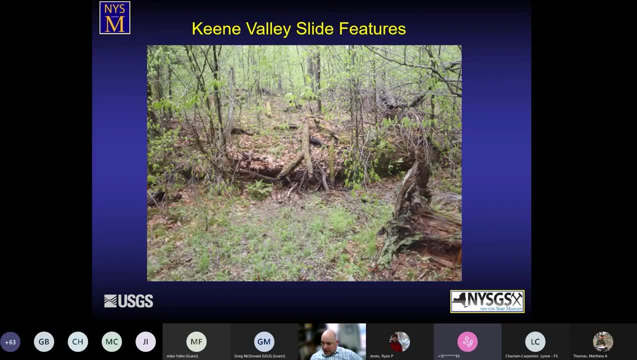 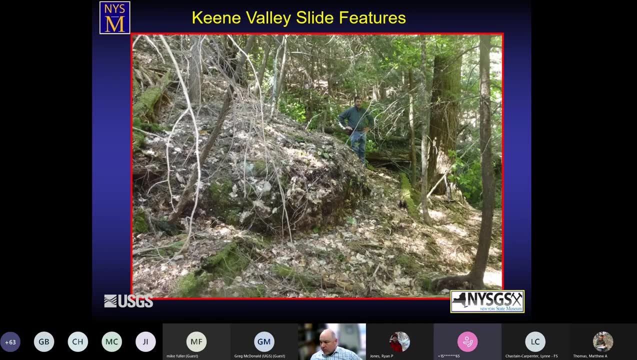 in the woods of the slide is creeping forward in uh late may to early june. again there's bill capella, the usgs, standing by an active portion of the toe moving through the woods. it was moving anywhere from five to six centimeters a day at first and then it's gradually slowing. so it was. 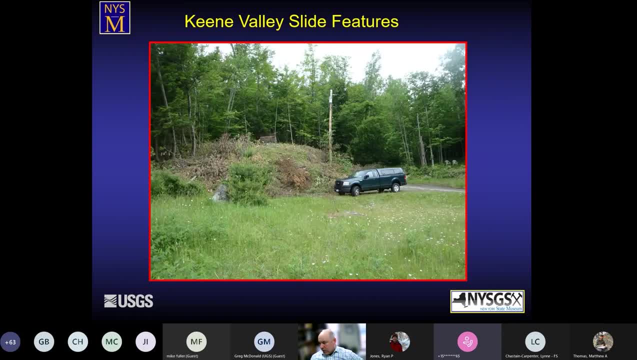 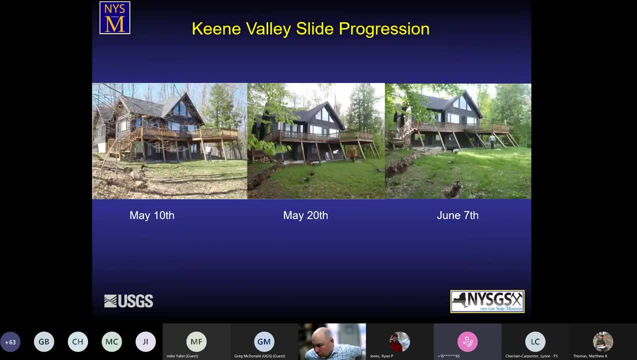 moving at a pretty decent clip. uh, early on, again, more pictures of the toe truck for scale, and there's a progression you can see on the slide of this house that was ultimately destroyed. uh, rotated sheared on multiple ends moving back down for scale. some other movement along the side where you can see that the foundation is buckling, and 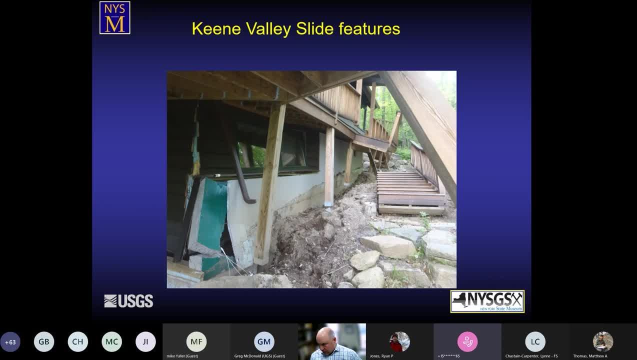 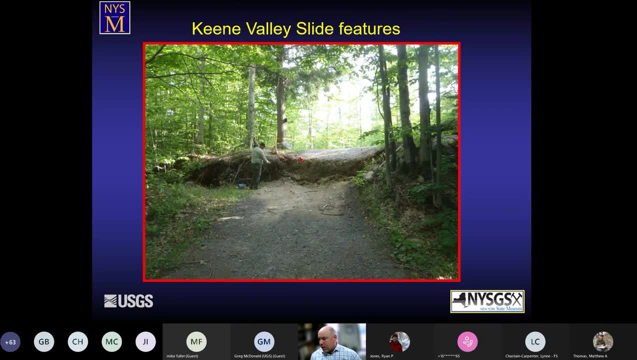 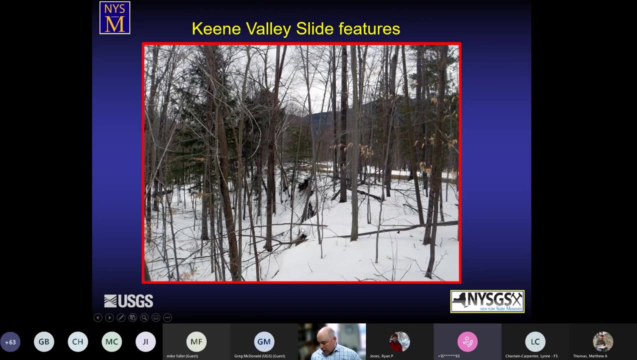 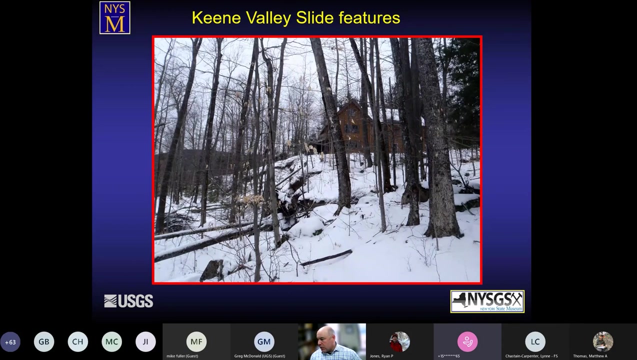 rotating and the actual pier's just crumbling. as this rotation, the slide continues downhill. that's the driveway to the house that ultimately was condemned again. the scarf here in the wintertime. you can see on the screen here, perhaps right there where the snow is breaking. another uh uh uh photo of the houses. these are large. 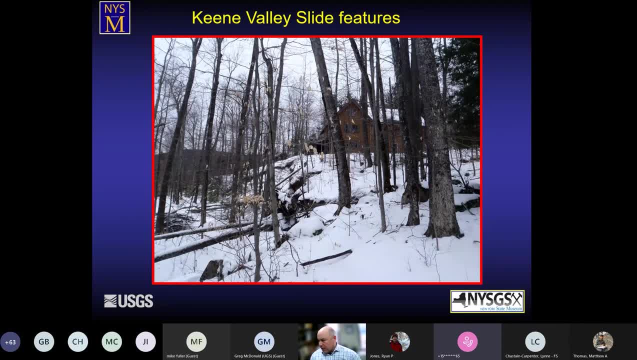 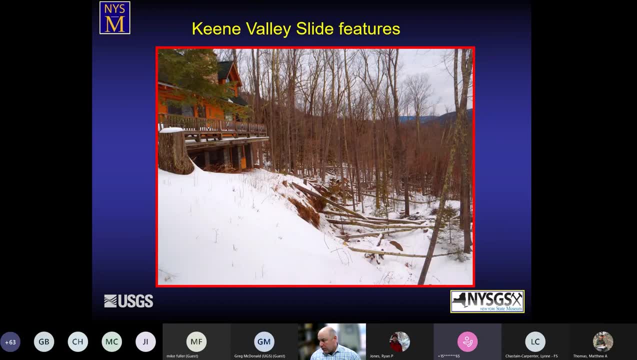 often mansion style homes. a lot of these people are from long island of city connecticut. they come up here and build these sort of staggering houses up in the very steep slopes of the mountains. um, again, another example of sort of the scarf that developed looking off towards giant mountain. 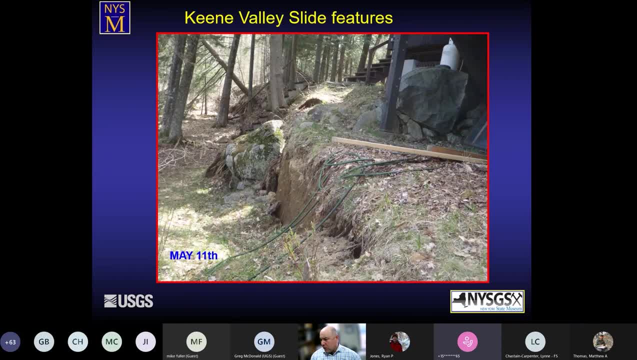 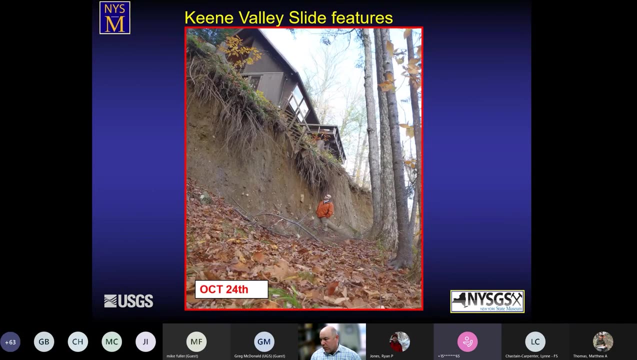 to the east and again, uh, some of the slides showing the propagation of this head scarf that developed. so this is may 11th. um, there's a set of stairs which will be referenced again in the future. here and again, this is october 24th. so, uh, this sort of slide really dropping and moving. 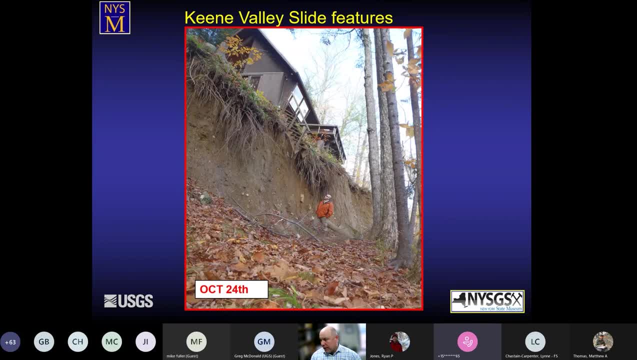 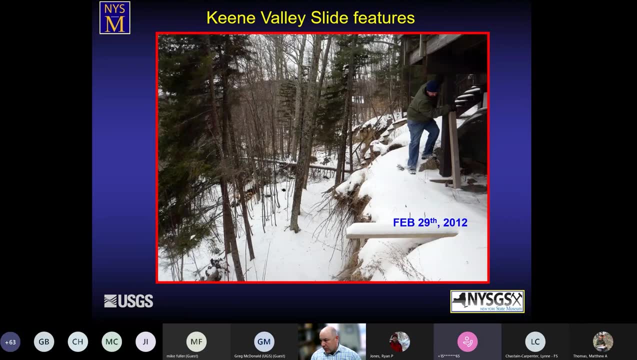 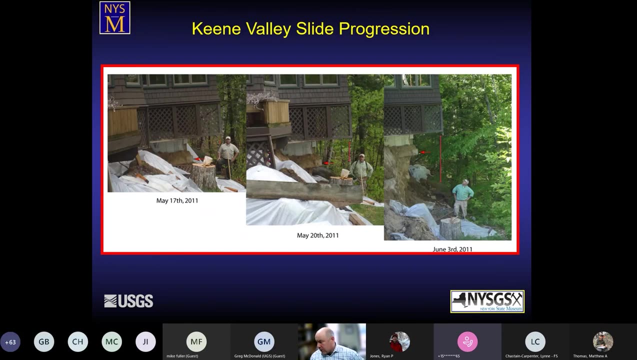 throughout the early summer months, when it was pretty active, and again february 29th of 2012- uh, seemingly somewhat stabilized this location again. other progressions- you can sort of see the foundation of the house here on this, this large scale house here dropping like a rock, literally um for june 3rd, and ultimately this ended up resulting in 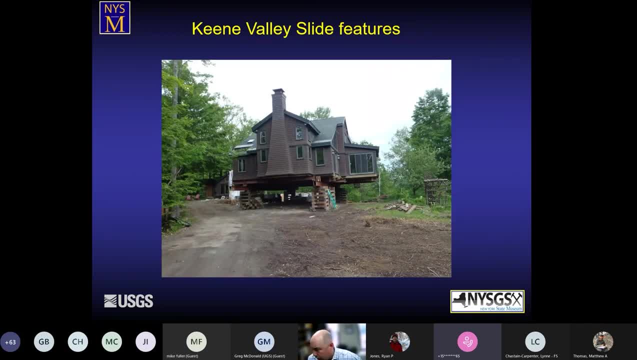 this particular location. this is a 3 800 square foot, what i would call a mansion or home. uh. that was ultimately picked up uh off of its uh foundation. the slide is right behind this house. this house was picked up. it was moved and relocated approximately 300 feet and set on a. 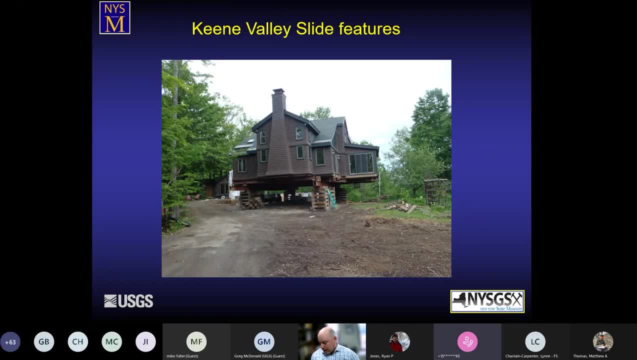 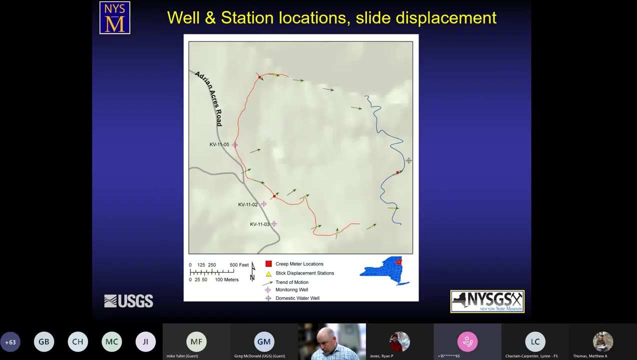 brand new foundation, um, uh, at the top of the property, um, so this is again 2011. uh, the house set on the new foundation. the house sold again in 2020 for 590 000. and again, just to map the overview of the slides and the slide footprints and sort of the directional vectors we picked up from sort, 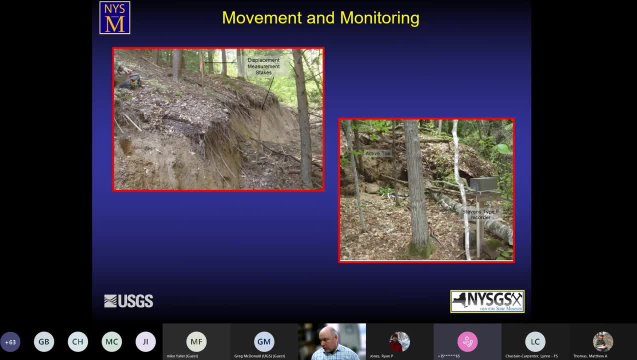 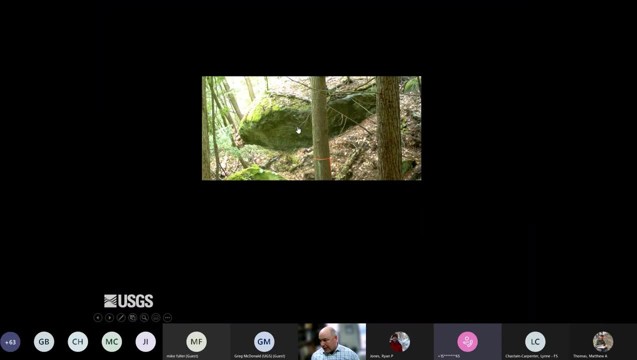 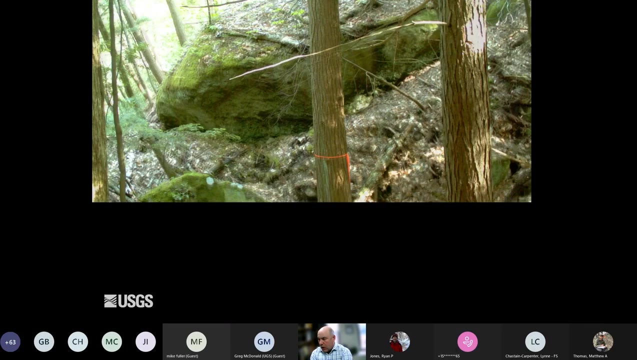 of some creep stations and other types of instrumentation we were using to sort of take crude measurements with along the lines um. this is a video we detected, we we collected, of movement on the slope, which hopefully you'll be able to see here again. moving down hill. we're off the slide, running a fixed object. 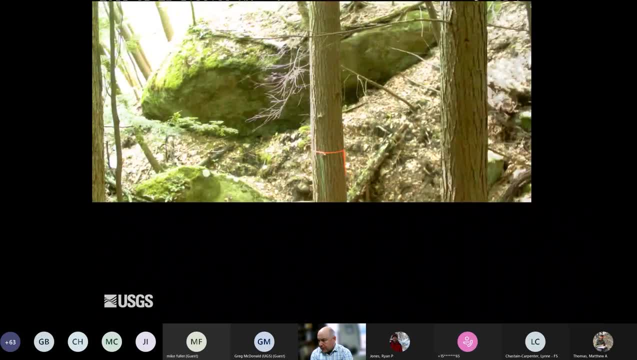 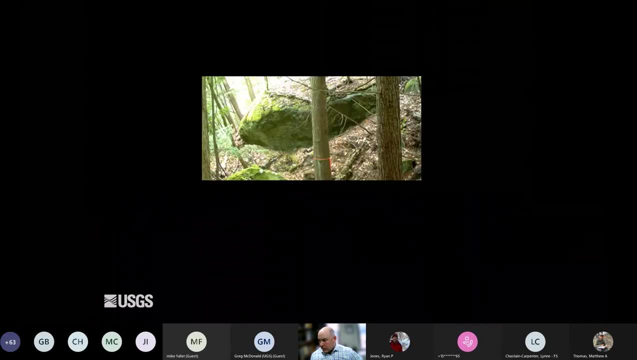 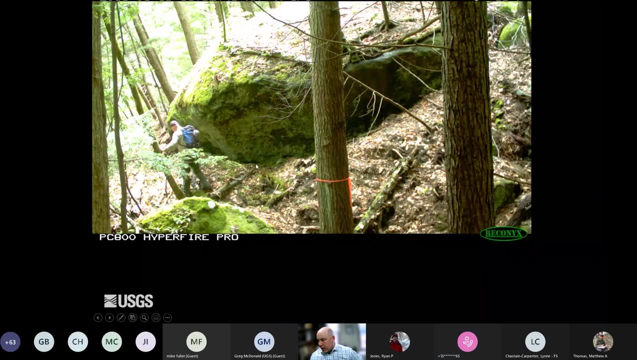 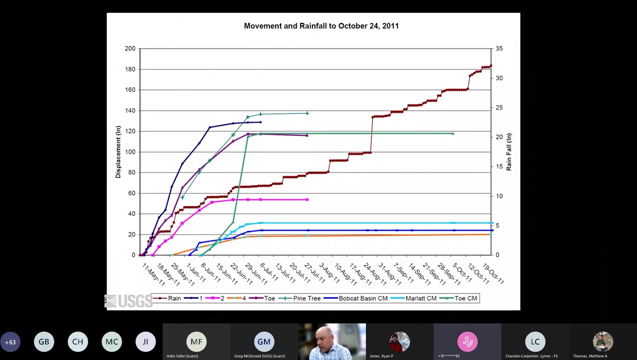 off the slide here, moving back through, creeping down slope. and there's my colleague again for scale, so very large boulders, very large sort of object again on this overall mass moving down slope to speak: um, these are our movements, including rainfall and movement sort of diagrams again, and one thing you'll see here is that early on again, 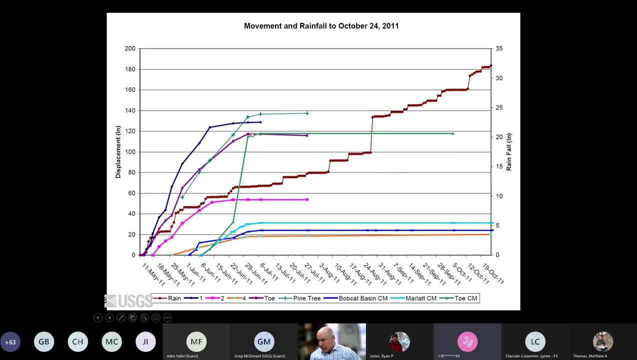 movement is sort of uh, raging pretty well and then, as we get right around this sort of first part of july again, overall movement starts to really decline, um, dramatically. you'll also see the brown curve, which has a pretty good stair step in it around the 31st of august in 2011. 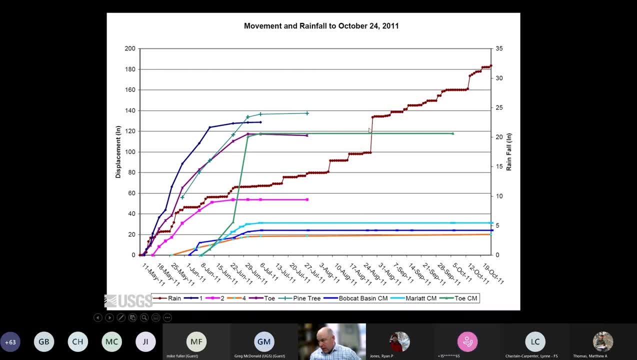 which is interesting again because that is a storm, uh, of pretty good magnitude that was associated with a hurricane. it came through the adirondacks and triggered dozens and dozens of debris, avalanches, but did not cause this slide to reactivate like we thought it was going to do. 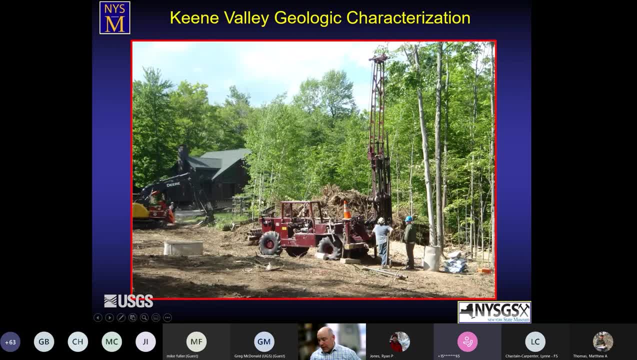 again, a lot of characterization on the upper parts where we could get access to the property again a mix of private and public property. the lower part of the slide was an area was purchased by developers that wanted to develop it and they did not want us operating or collecting data down on the lower slopes. 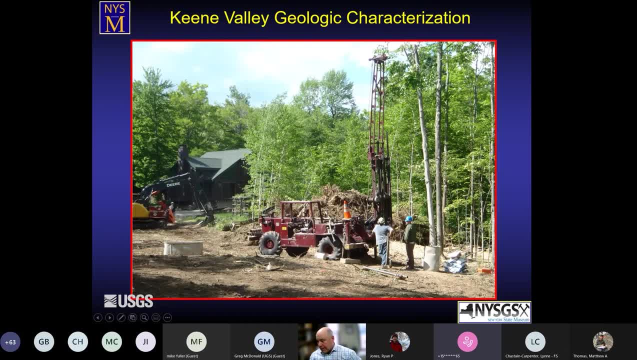 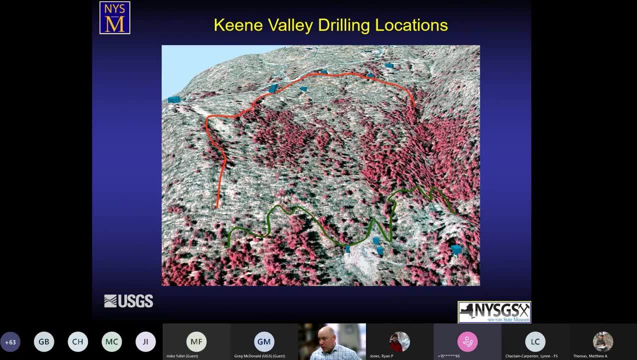 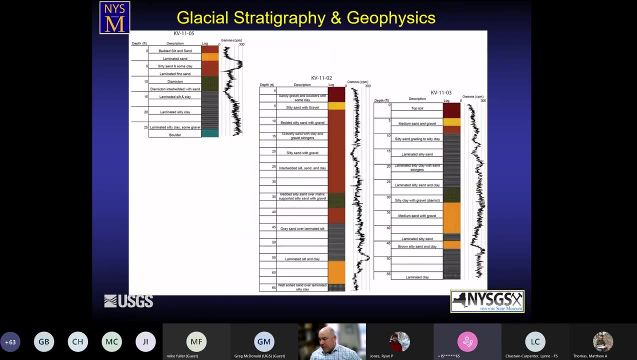 so we would only be able to work where landowners would give us permission and the one or help sort of gauge what was going on if their houses were going to sort of make it. so some over locations, again, monitoring walls were installed to monitor groundwater levels. just again, the characterization of this and then our overall net characterization. so 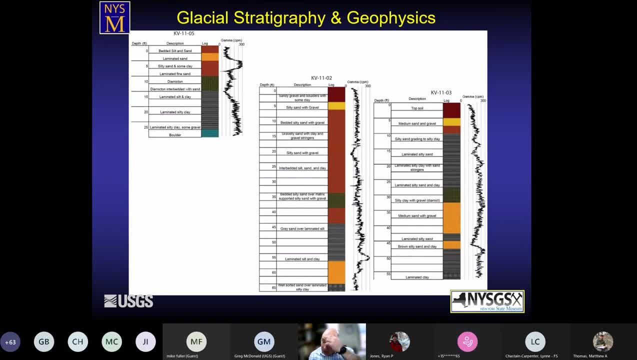 despite being able to see bedrock almost in every direction, we were able to see entire property um in this location, and so at that time, if we were able to observe soil conditions or check soil conditions, that might be a lot more complicated. if we were able to see what the soil conditions were, and what the soil conditions were, we would have. 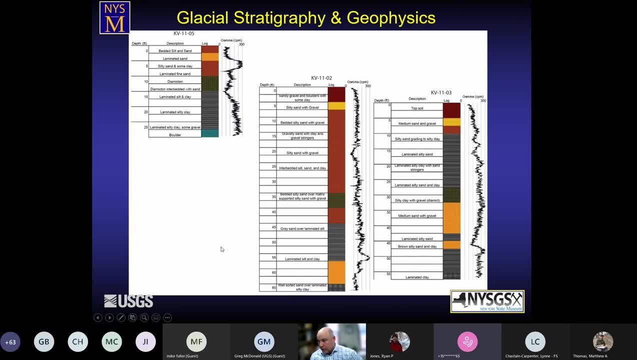 tried to identify what was going on in the soil. uh, there was a lot of space in this construction section of the slabs of 65 feet with holostem augers and then basically could not get any further down if drilling conditions became difficult. there was concerns about uh doing some sort of 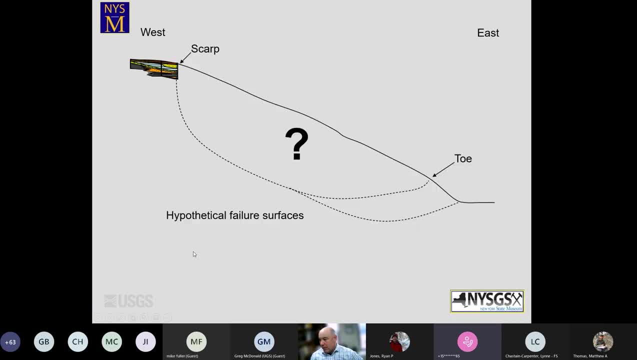 wells. But just to put this into perspective, this is again compared to what the overall slide was in its overall dimension, showing a hypothetical failure surface. There was an older, very deep well at the bottom of the slope that we had access to initially. Eventually we lost. 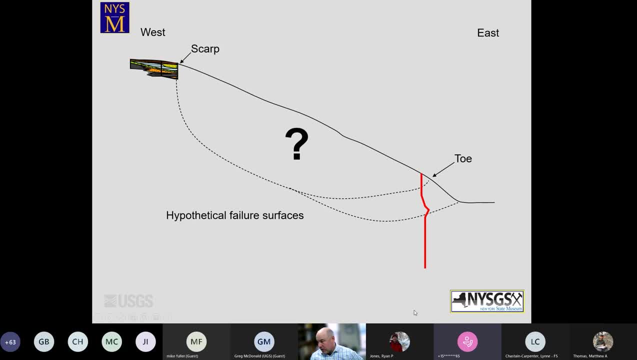 access to it because the kink from the slide caused the casing to shear so much. But we could measure the location of the sheared well casing to estimate where that shear surface came out down below. But again we're unable to collect any subsurface information on the actual failure. 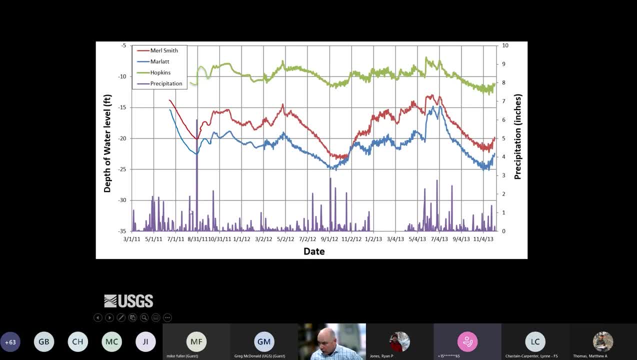 itself. So this is our groundwater level measurements. We monitored this for about three to five years after the slide, when it started again- And this is the Hurricane Irene again around August 31st- Again, really quite a storm. We really imagined it was going to reactivate the. 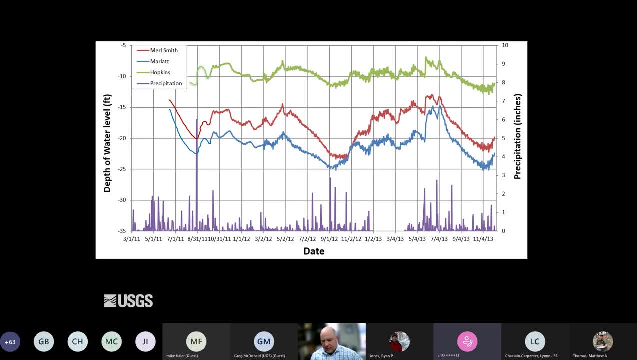 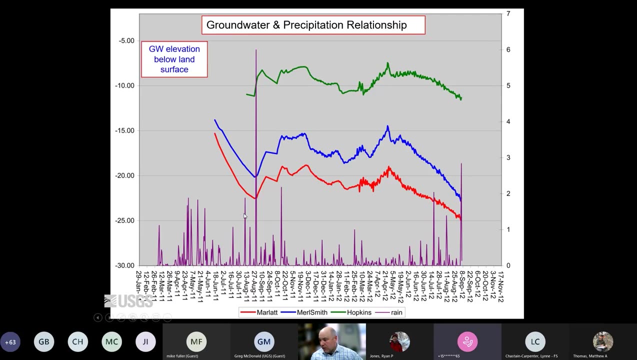 landslide that didn't, which is kind of fascinating for us because it's got obviously some very complex sort of groundwater trigger mechanism going on that we were never able to fully quite deduce in this location. And again, just showing again the overall groundwater elevation levels and 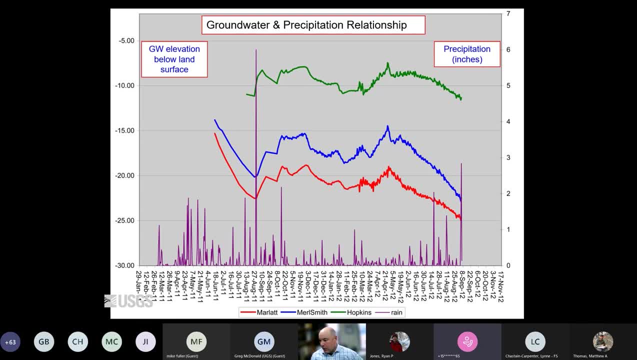 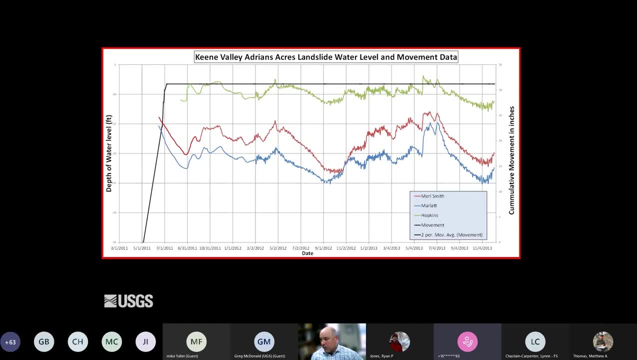 precipitation events, sort of the storm of record coming through at this location. that did not reactivate the slide. So again movement, water table, so on and so forth in this slide. Ultimately we ended up doing surficial geologic mapping again in the Keene. 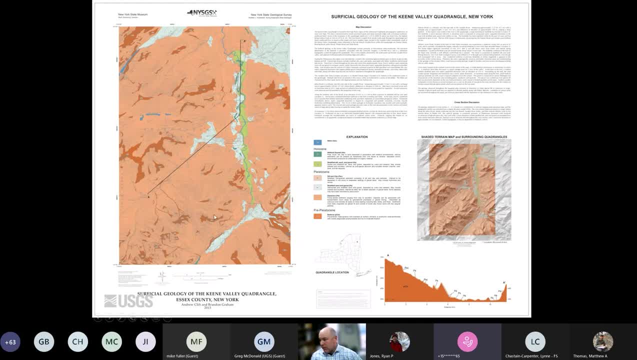 Valley Quadrangle as part of our solution to sort of address the situation And we did a lot of work on the geological map to sort of get the best of it. We did a lot of work on the geological map system- provide some additional information for the local planners. There's the map itself and cross 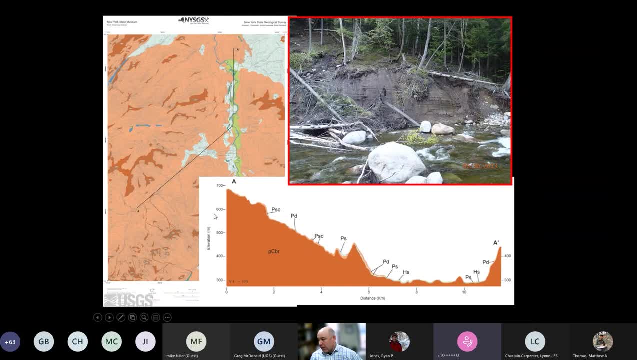 sections. Again, one of the things that was discovered as we continued upstream in these mountain streams are that even locations that were really really high, much higher than ever before, believed to have been able to contain sort of proglacial lake sediments we would commonly 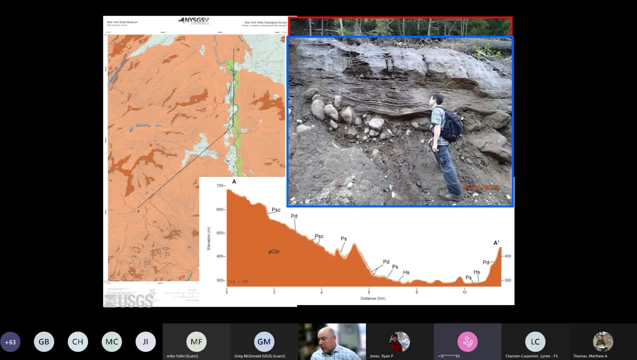 find laminated proglacial lake sediments. high up in the mountains, right in sort of the edge of the high peaks, There's some of these laminated lake clays that are overlying sort of the mountain. So there's some sort of alluvial boulders, probably from a pre-glacial timeframe, something along those. 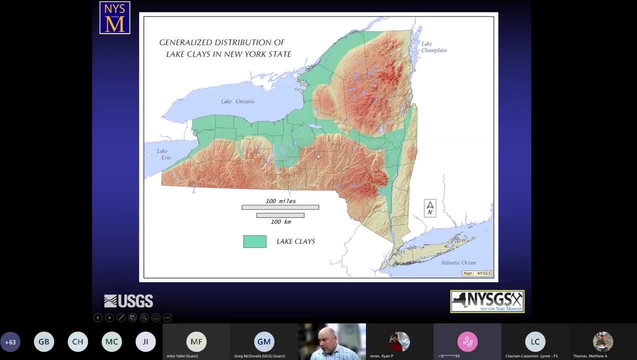 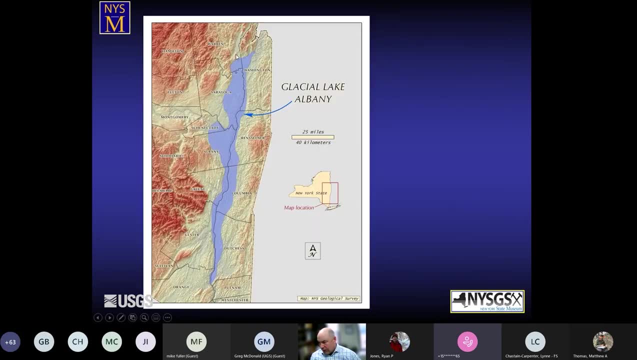 lines. So again moving back to the lake clays, that was the Adirondack story, And then now look at this generalized lake clays throughout New York State. looking back a little more detail in the Hudson River Valley where we had Glacial Lake Albany, which was again extensive throughout the 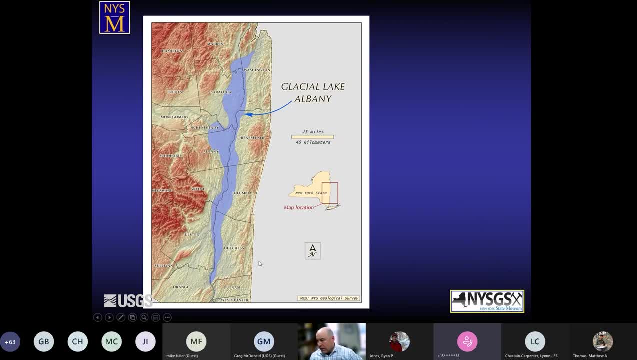 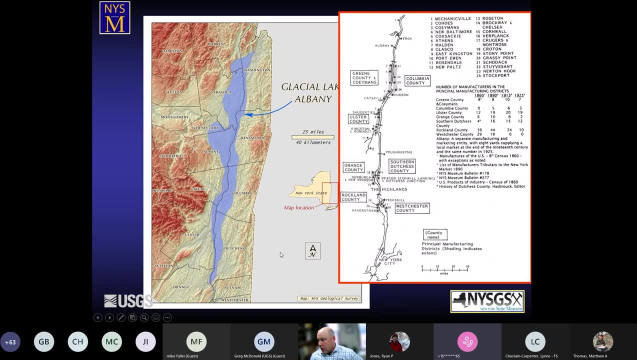 Hudson Valley and has affected locations in Albany and Troy- Those are the two major cities here in the Capital District- and Schenectady. At one point in time there were 131 brick yards operating within the Hudson River Valley. Back in the 1800s it was the. 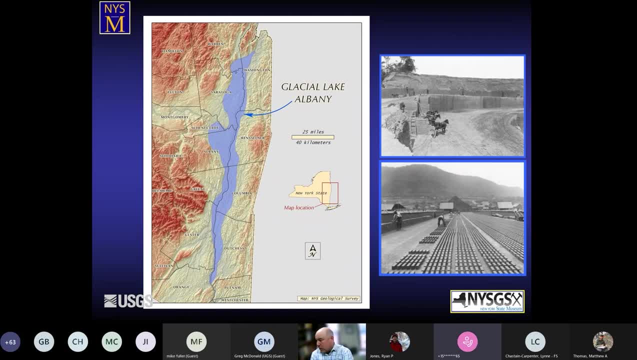 principal source for bricks in the Northeast. So some old photos showing how it was done back in the day with horse and cart. They laid the bricks out in the day and let them dry for three or four hours before they got them off the kilns And sort of a very labor-intensive process. And this was also 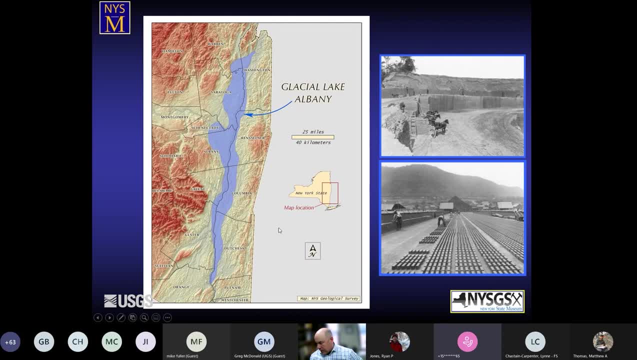 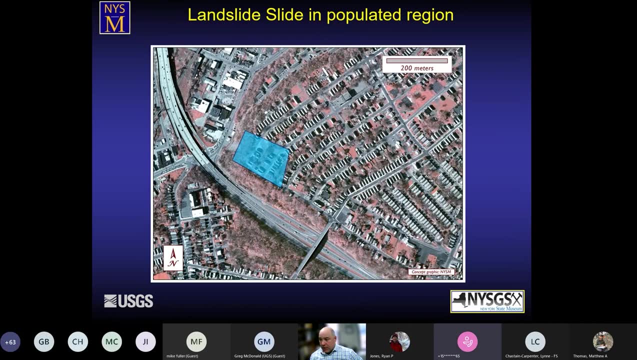 an outcome, largely because New York City kept burning. I think it burned down three times before they started to mandate the use of bricks as a construction material. So there's your sort of an urban photo, again of a populated area The blue rectangle represents. 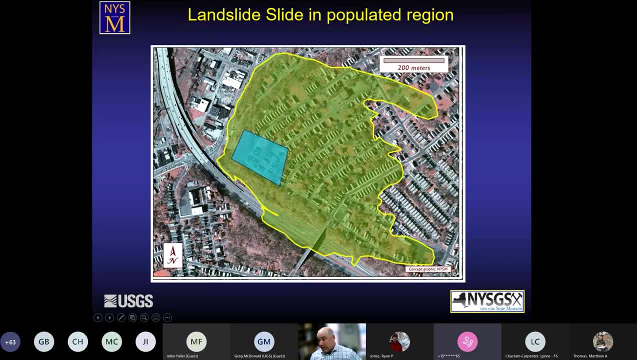 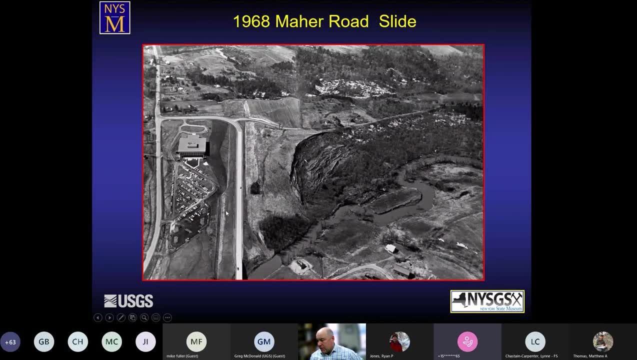 a typical-sized two-acre or so landslide, Just for example, that's the Keene Valley landslide by comparison And just as an example again of our slides that we see down here in the Hudson Valley and these lake clays. they're large, often multiple rotational failures. This is 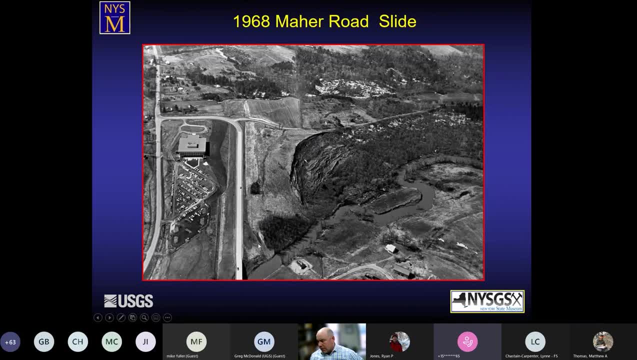 the 68 Mahar Road slide along the Normanskill River, which is a stream system that's been sort of rising itself through these glacial lake clays and silts since Lake Albany drained. The time of drainage of Lake Albany is not exactly well pinned down. There's cars for scale buildings, The 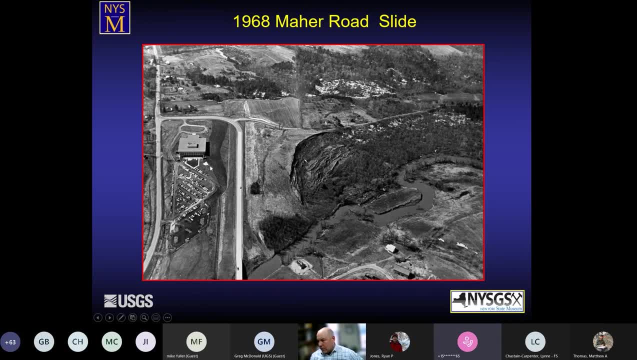 building you see in this photograph on the left was abandoned probably 15 years ago And we don't know exactly why it's still for sale today, but we suspect there may have been foundation issues that were noticed and it was put up for sale and has not been resold, sitting there, vacant to this. 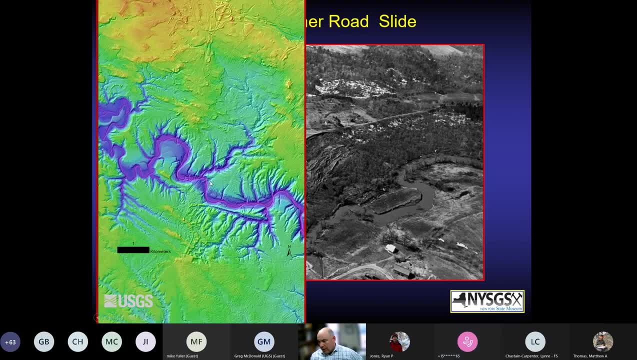 day And again some nice LIDAR imagery showing the Normanskill River and the location of that slide from Mahar Road And again lots of these steep meander bends. Some places we have 10 to 50 feet of sand, often dune sand that has developed and blown over, So there's dunes up on the upper part. 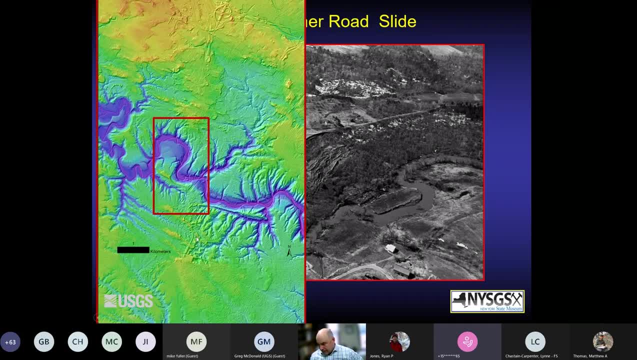 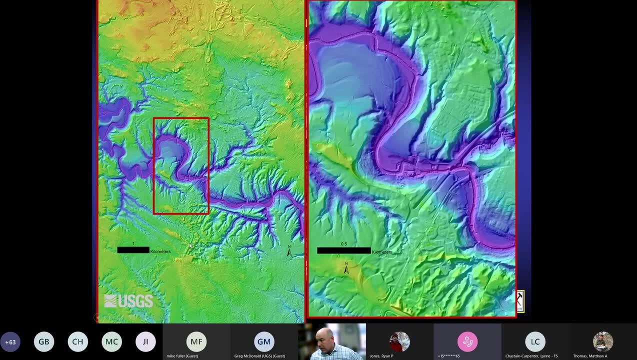 of this LIDAR image that have overlain, which is nice. The sand itself drains until you get into the lake clays that are underlying everything. There's a close-up of the Mahar Road slant Mahar Road slide. over here to the left of the main road. you can see other slides taking place as well. 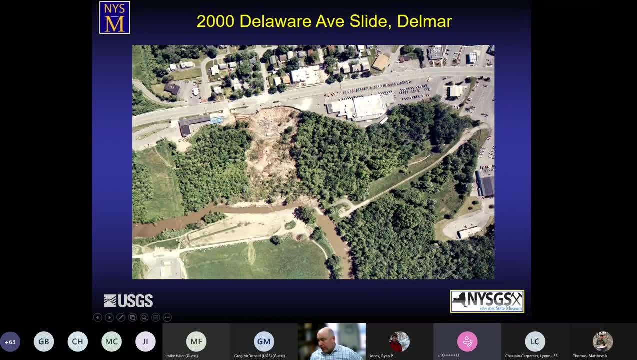 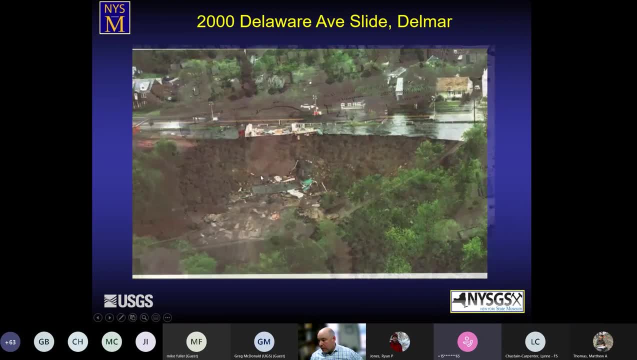 On Delaware Avenue in 2000,. another large slide of these glacial lake clays that shut down, ultimately Again, State Route 443, which is a main artery into the city of Albany. Until it could be rebuilt, there was a building and a vegetable stand and a parking lot that 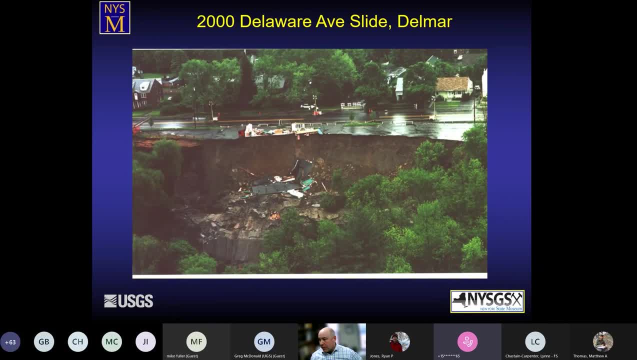 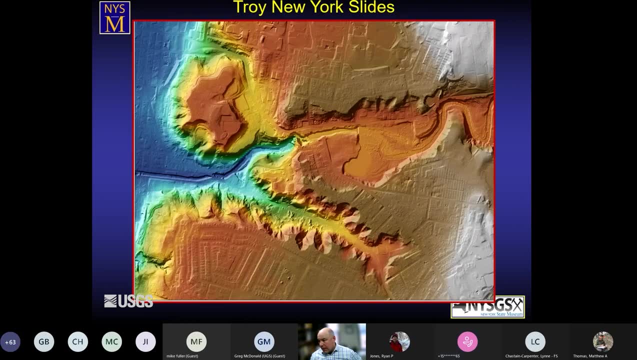 was lost. no fatalities, fortunately, in this location. These are exceptionally common here in the capital district, in these glacial lake clays and also in the Hudson River Valley. Here's a LiDAR image of Troy, New York, showing you can see that the population density is very 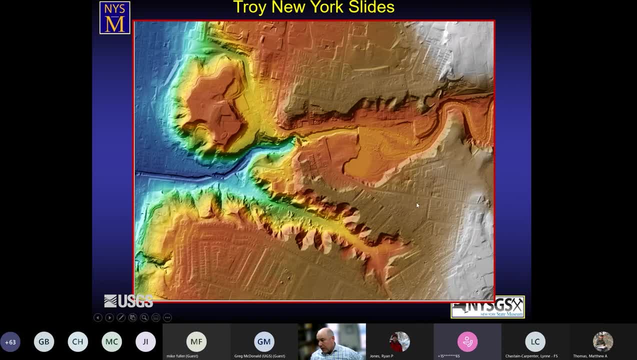 built up on these lake clays throughout the Hudson Valley. This is the location, right there, of the 1843 Mount Ida landslide that was responsible for 17 deaths in that particular slide, And then in 2011,, during Hurricane Irene, the same hurricane I mentioned to you folks. 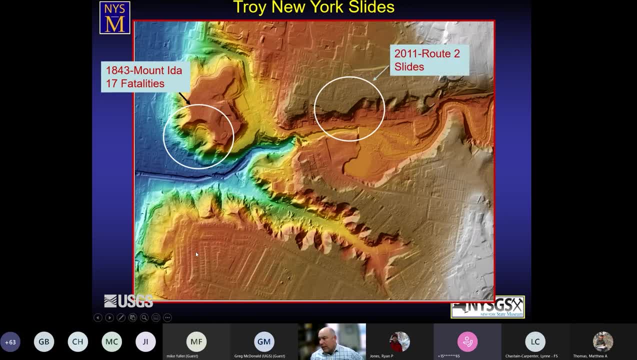 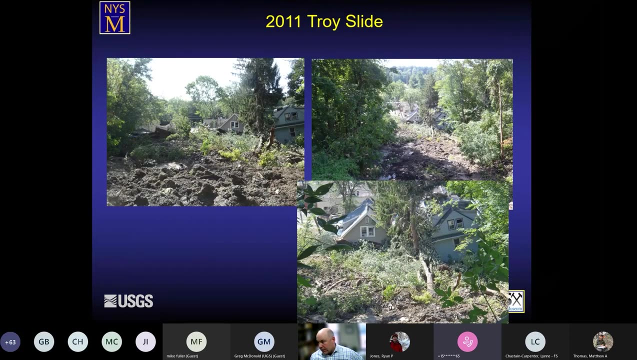 earlier for the Adirondacks triggered a number of landslides along Route 2,, again in these glacial lacustrine clays which have been built over, and the result was the loss of numerous houses from these sort of rotational failures, moving back down on the landscape. 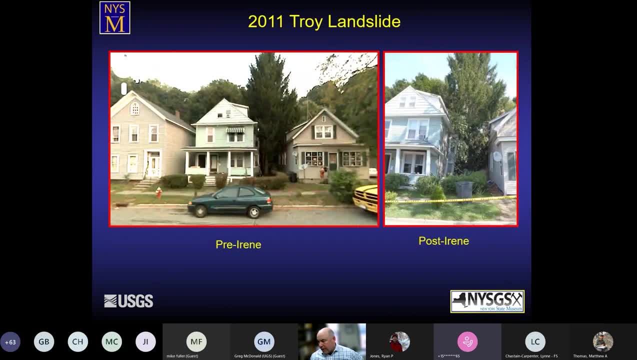 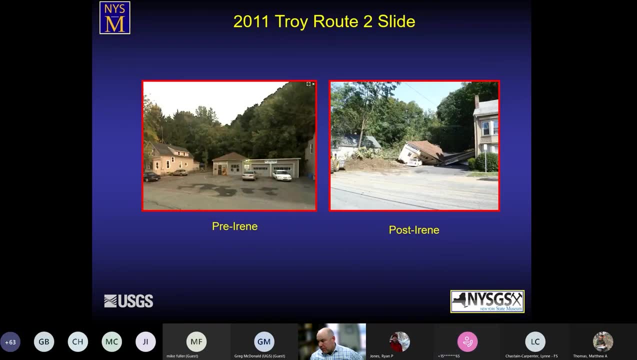 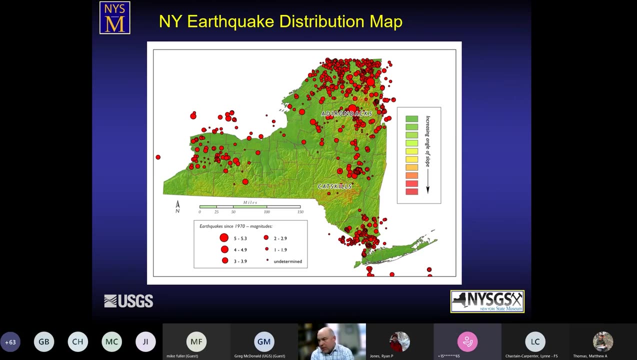 So some other slides showing pre-Irene Hurricane, Irene, post-Irene house depletion, Displacements on the landscape, so on and so forth. So another factor that is sort of makes me a little bit nervous about things is the distribution of overall earthquake activity. 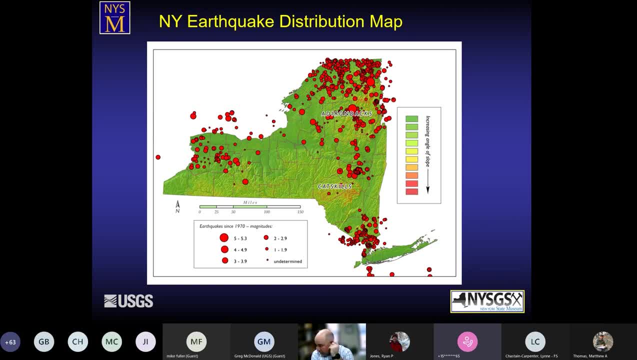 We don't have a lot of very large-scale earthquakes, particularly like the folks in California who had sleep through almost all of these, but we have enough. We have sort of one documented landslide triggered by some seismic activity, but I think it's really just been a. 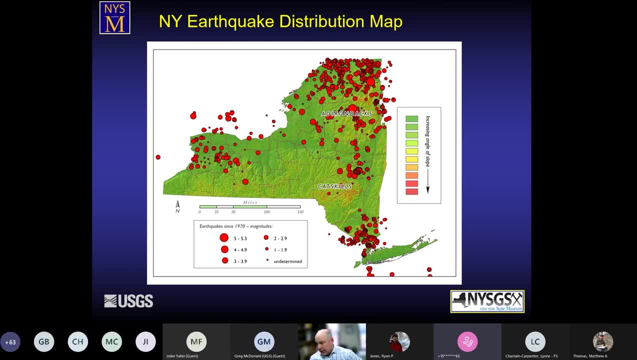 matter of looking at it, And I think it's really just been a matter of looking at it. So one of the things that you know I thought about when we were doing the work in Keene Valley and some of the work that's been done also in the Hudson Valley, is a lot of our landslides end up. 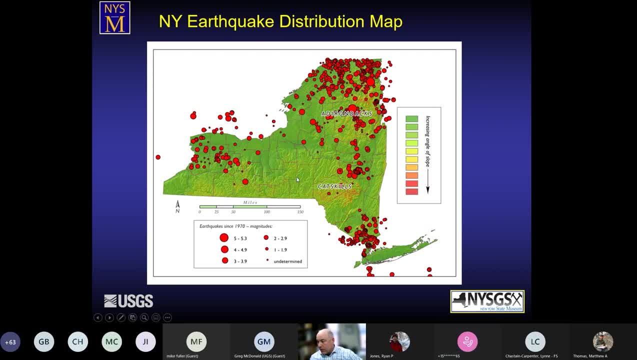 happening at sort of when we have the end of winter, March, April, right, The snowpack has been melting off groundwater's super saturated. Maybe we'll have a large-scale rain on snow event. And you know, to my mind it's always wondered if we ever had a decent seismic pop at the end. of March or the first part of April in the Hudson Valley. So I think it's really just been a matter of looking at it And I think it's really just been a matter of looking at it. And I think it's really just been a matter of looking at it And I think it's really just been a matter of looking at it. 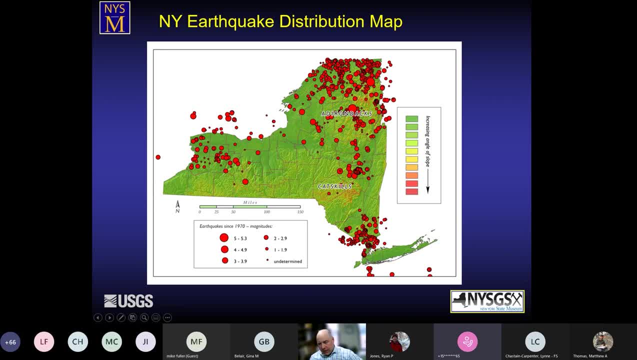 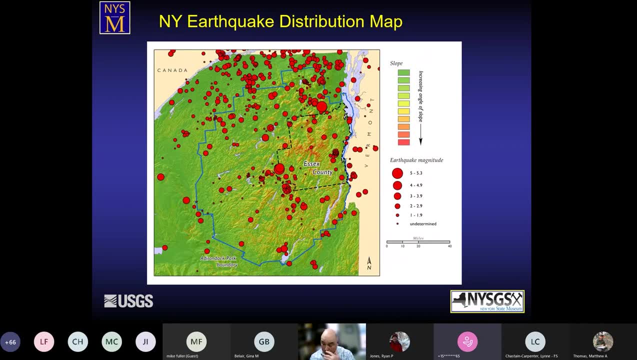 Hudson Valley down the New York City area. you know that could be very bad given the distribution of lake clays we have in New York State for large areas. So I think that's been a potential trigger mechanism that we will just dodge the bullet here for a long time and hope we 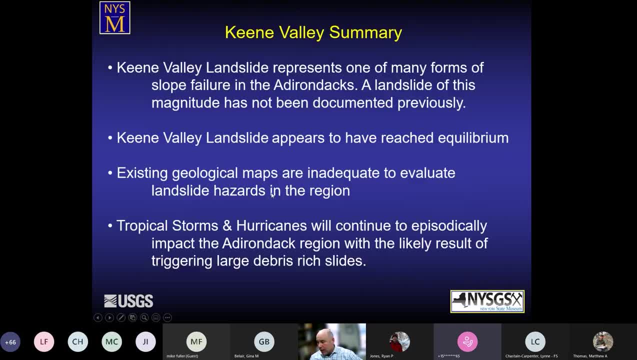 do continue to do that. But again, I think additional surface geologic mapping would be helpful for that. So sort of in summary, again, the Keene Valley landslide represents sort of one of many types of slope failures we've seen in the Adirondacks And I think it's really just been a potential trigger mechanism that we will just dodge the bullet here for a long time and hope we do continue to do that. But again, I think it's really just been a potential trigger mechanism that we will continue to do that. But again I think it's really just been a potential trigger mechanism that we've 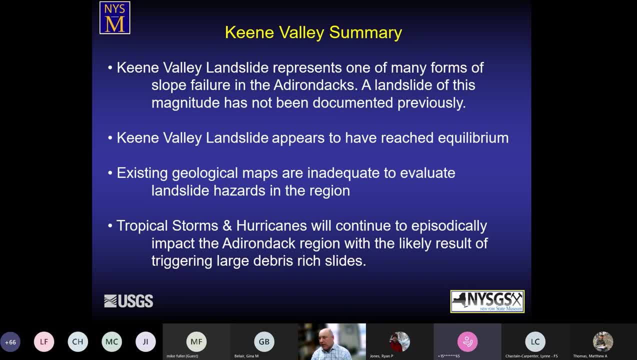 got a slow-moving juggernaut style, triggered by some combination of snow pack and groundwater movement. We later on discovered by some of the landowners that the houses up there have a collective singular well that puts water into a large cistern And that well and that cistern. then